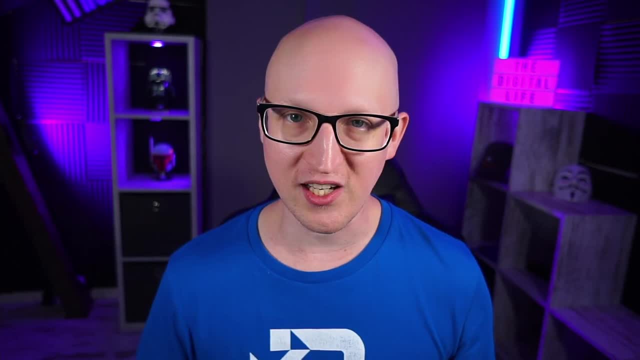 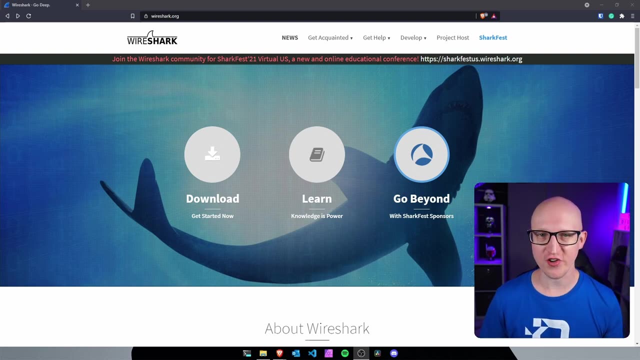 But here we will cover the most important features everybody will need. So let's just get started. Wireshark is a free and open-source packet analyzer. It is the absolute gold standard across many companies and used by nearly every network or security guy. So whenever you want, 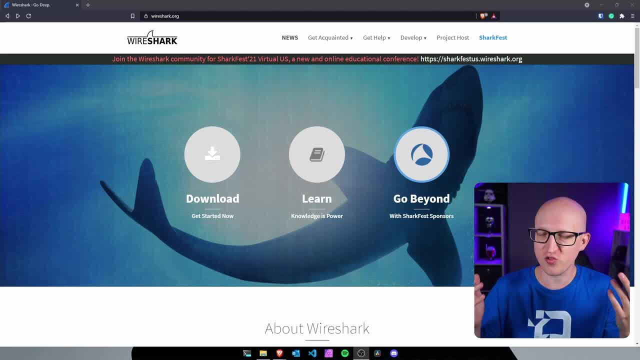 to analyze network packets, troubleshoot issues or just do it for education or researching. Wireshark is the tool that you're going to be using. It can capture network packets that are sent to the network card of your computer, And you can also import packet captures that you have created on other machines as well. 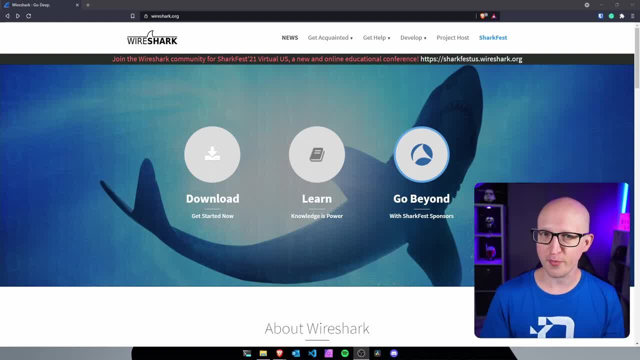 And it allows you to inspect all the details of these raw network packets that are captured, and it also interprets them, So it automatically detects certain aspects of the packet, just like ports, protocols and many other things. you can easily follow and understand what's going on. You can download it from the official homepage. 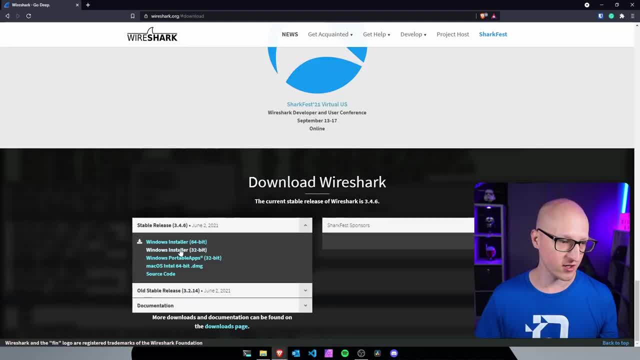 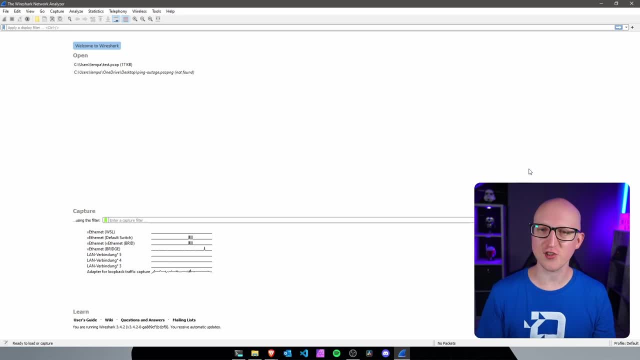 Wiresharkcom And just click on download, and then you can install that on Windows, Linux and of course also Mac OS. This is Wireshark when you open it the first time And before we can actually start capturing network packets, you need to select your network card interface. 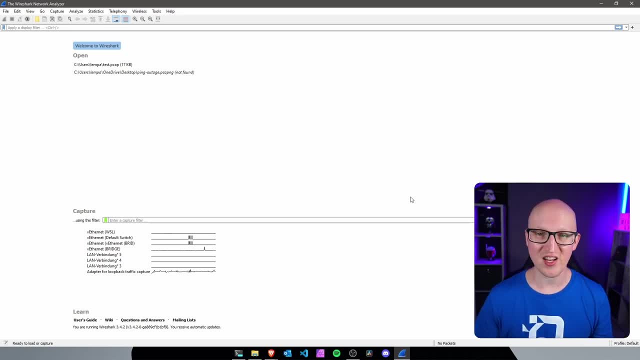 So, depending on your setup, that usually shows up any wireless adapters, Ethernet cards and etc. So in my case, you can see, I have many network card interfaces And this is because I also have some virtual machines on my Windows PC, just like the Windows subsystem for Linux, I have a default. 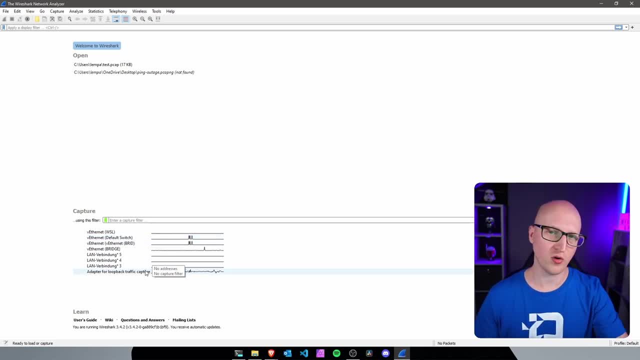 switch for my Hyper-V machines and also my VPN connectors for Tailscale and whatever. So first of all, you need to identify your main network card interface, usually your physical network card or your wireless adapter. you want to capture any network packets. In my case, 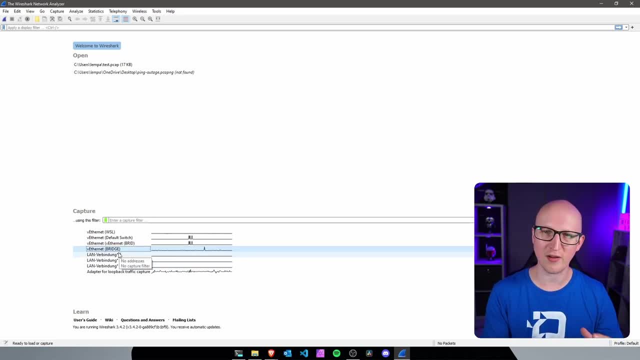 it is the VEthernet bridge, And this is a virtual bridge between my physical network card interface and a virtual switch for all my virtual machines, right So when I select this and I can start capturing all network packets by just doing a double click or selecting it and click. 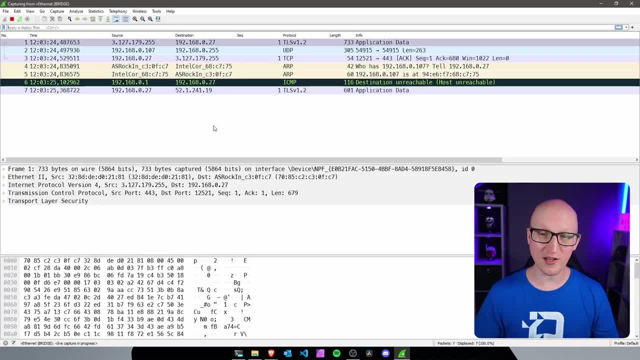 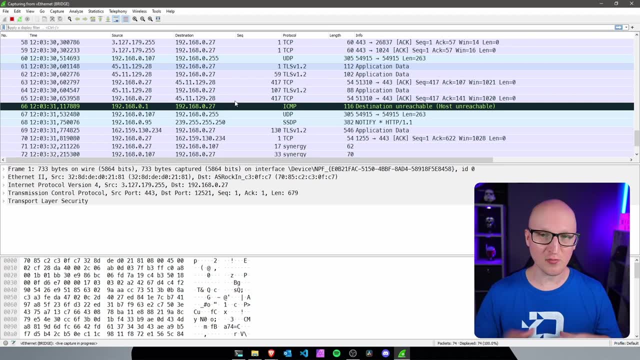 the blue icon on the top bar. So let's click on that and it automatically starts capturing all the network packets that are going in or sent out by my network card interface, And you can see it captures a lot. So there's a lot of stuff going on in the background usually, So when you click. 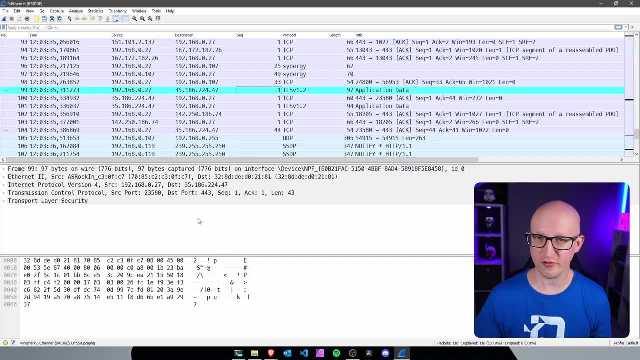 on a specific network packet, you can inspect all the details of that packet and read everything, for example the MAC address, the IP address, the ports and also the data that is sent over the network card. But before we step into analyzing the network packets and how to see IP addresses, 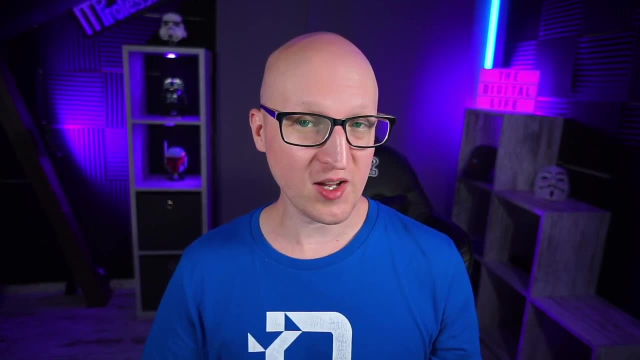 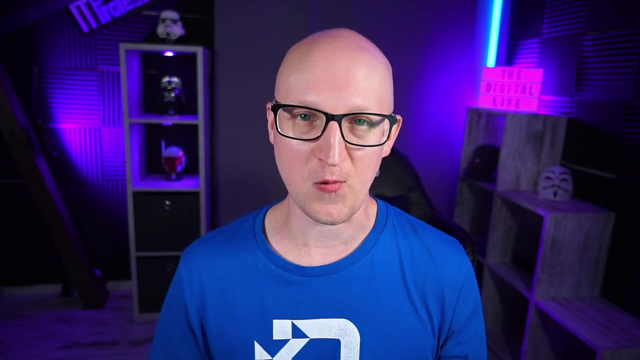 ports, traffic streams, etc. let's take one step back and talk a little bit about network basics, Because if you don't understand networking, it will be fairly hard to use a tool like Wireshark. By the way, if you want to learn networking, the COMTA Network Plus and also the Cisco CCNA. 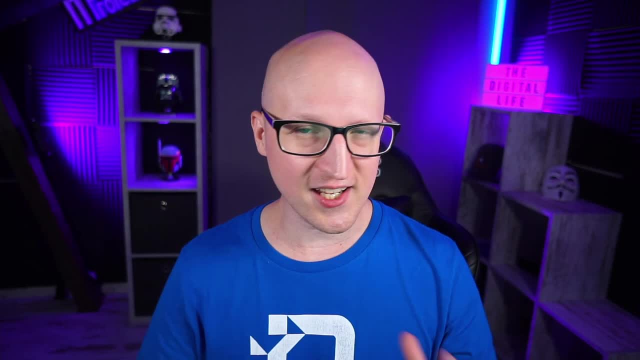 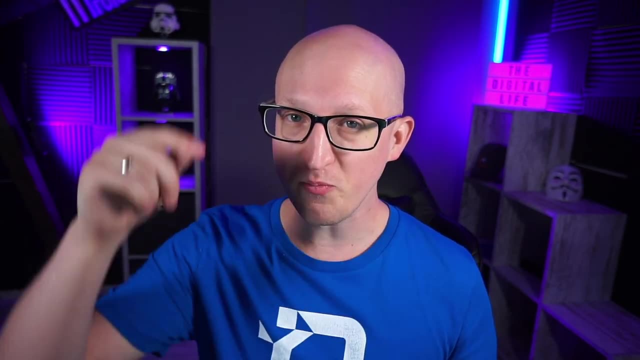 are both really great and valuable IT certifications for any IT professional. So if you're searching for great training courses on them, then check out ITProTV. for example, With the link in the description down below, you will get 30% of all subscription plans from ITProTV forever, So just check it out. 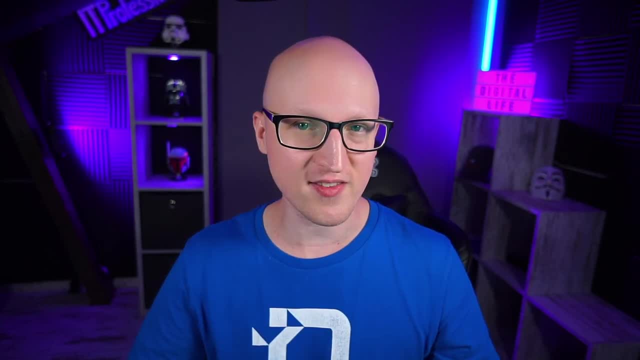 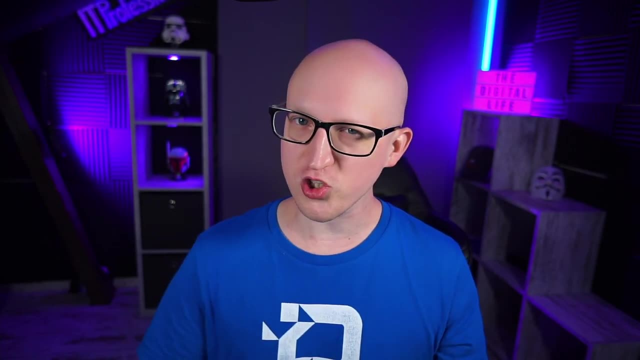 Okay. so as I said, in Wireshark we only capture network packets that are sent out or received on the specific network card. We do the capture. So in any wired network we usually only see packets for our PC and not for other devices in the network. 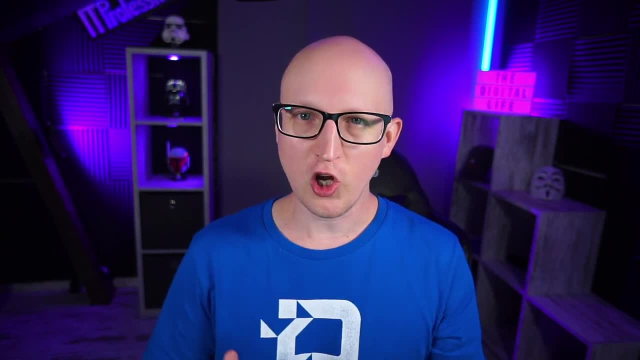 That was a bit different back in the days when we had hubs, But nowadays network switches are smart enough to know on which Ethernet ports our PC is connected and it will only see packets for other devices in the network. So in Wi-Fi networks this is a little bit different, of course, because every device 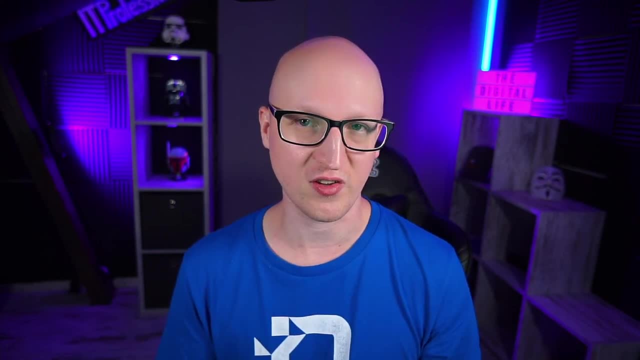 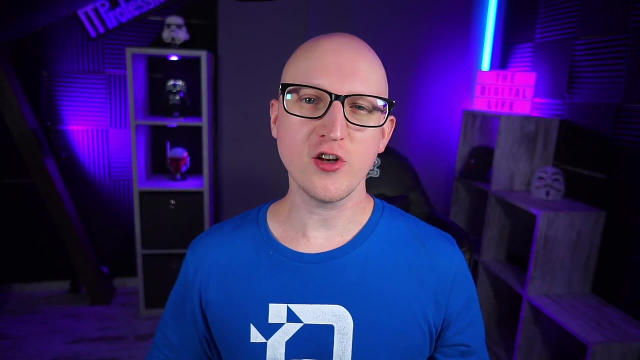 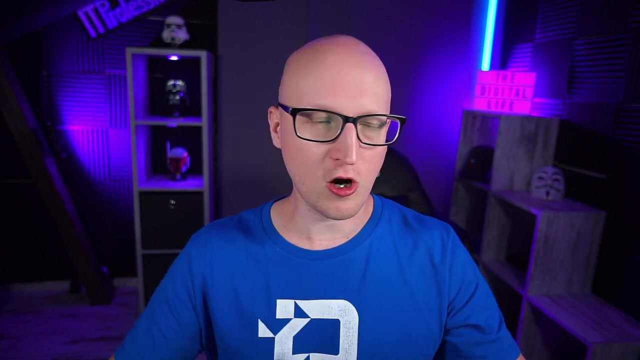 that gets the radio signal can also technically capture these packets, So that's an important thing to keep in mind. If you want to capture network packets for other devices within your network, then you should always make sure that you're capturing it at the right point in the network topology, So, for example, on gateways, where all traffic 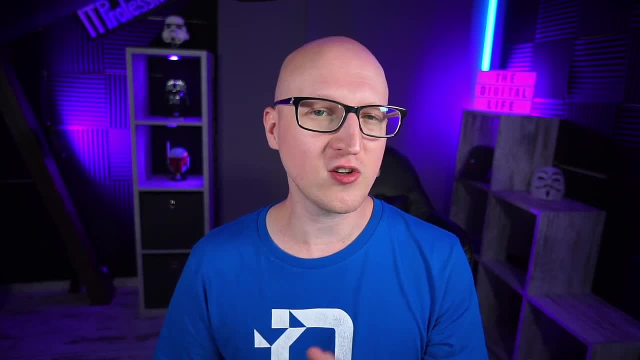 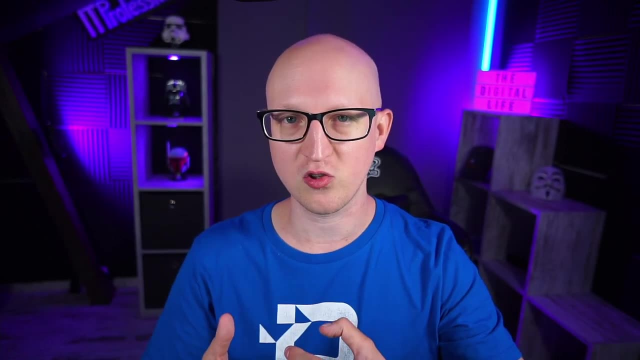 is passing through, or servers or clients where you're expecting to receive certain network packets. I will later explain how to create packet captures on remote Linux servers and how to import them into Wireshark to analyze them. That's very helpful if you want to check whether 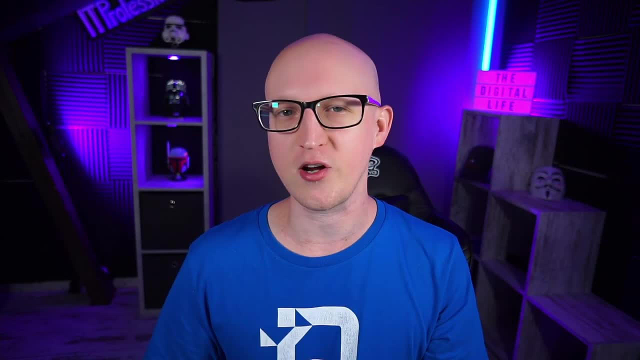 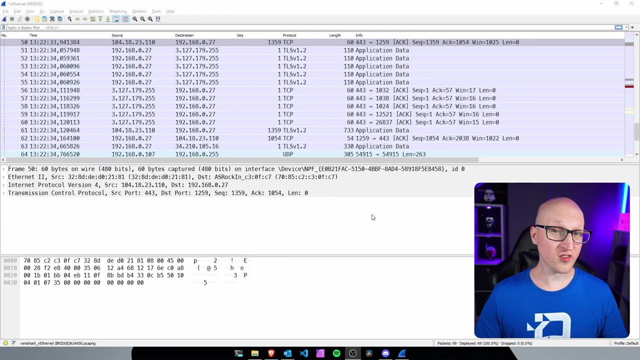 traffic is going through a specific gateway interface or VPN network, But for now we are capturing only network traffic that is hitting the physical network card of my PC. Okay, so let's start capturing actually useful information, For example, something like a DNS request. To start a new capture, we can just click on the same icon. 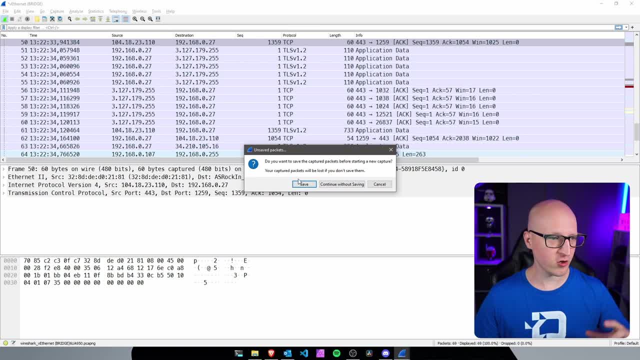 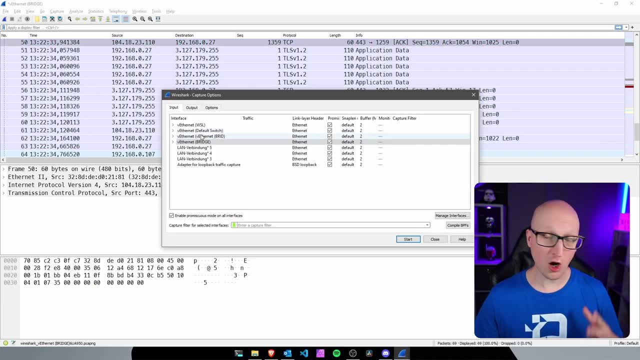 and it will ask us if we want to continue without a saving or if we want to save our current packet capture to a text-based file. But we can also do something else. For example, click on capture options to select a different network card interface you want to capture on And we can. 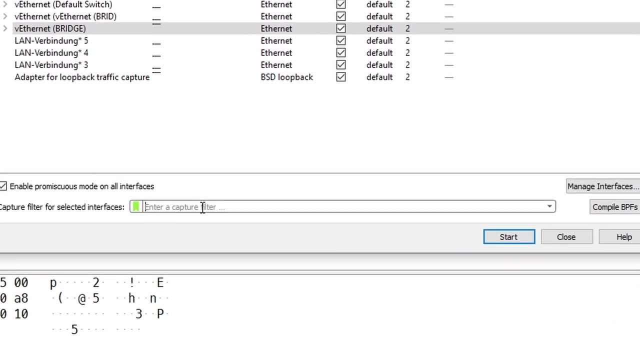 also apply a capture filter here. So, for example, if you only want to see ICMP packets here, or we want to capture the traffic between our PC and a specifically new server by entering the IP address here, So note this will only capture any network packets that are in the network card. 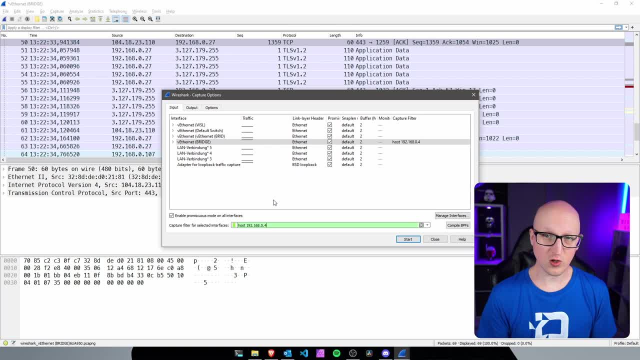 Where the filter applies to, So you won't be able to capture anything else, even if it's hitting the interface. So this can be very useful to shrink down the size of the packet capture file. For example, I was once doing packet captures on big data center gateways where 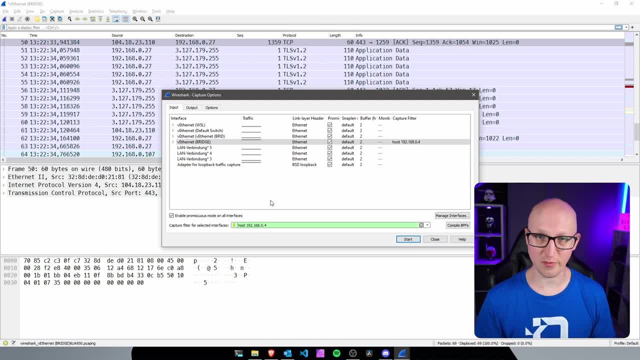 those files get really, really large in a very short amount of time. For example, every second it grows in a few gigabytes. right In this kind of situation it can make sense to shrink down the size by only inspecting specific protocols or specific 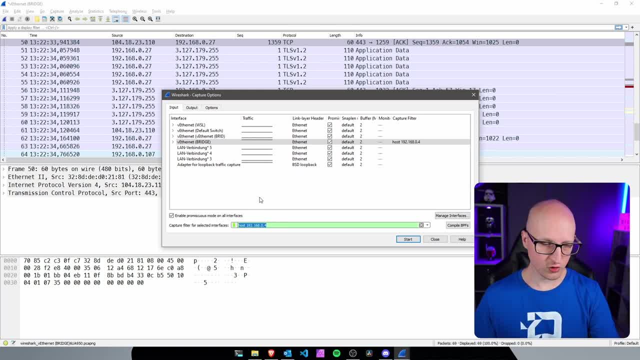 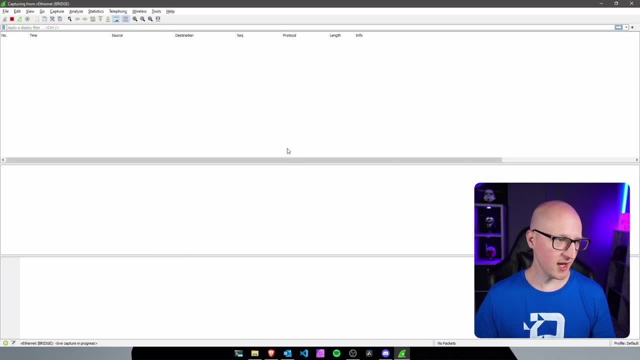 IP addresses. But on a normal PC you usually can capture everything here and filter it later in Wireshark. So let's start another capture and actually try to do some DNS requests and analyze them. So, for example, let me open a new 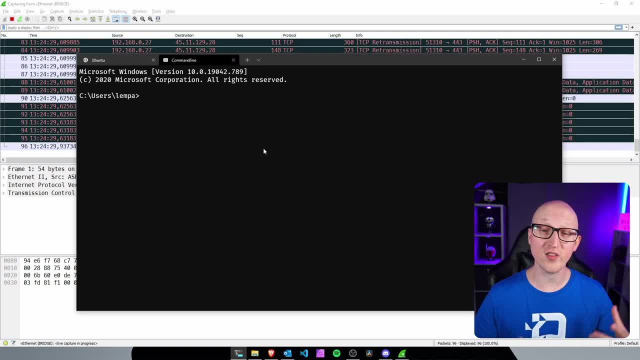 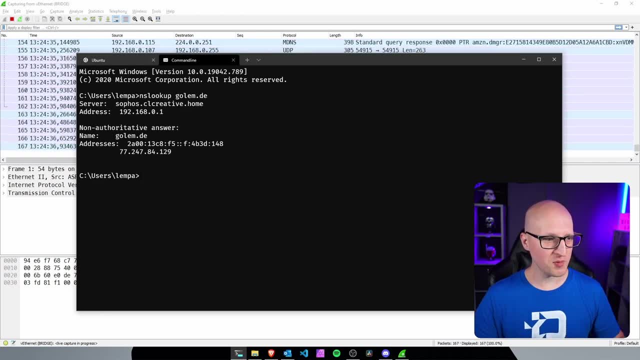 terminal here and I will use my Windows PC to generate some DNS requests. For example, let's do an NSLOOKUP to golemde And when I hit enter, my PC will generate a DNS request to my primary DNS server that I've configured, in this case Sophosclcreativehome, and the server will. 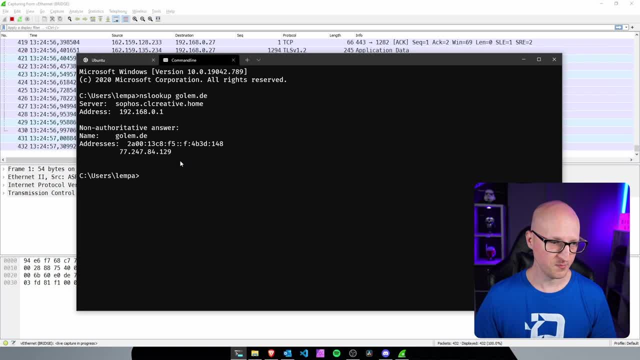 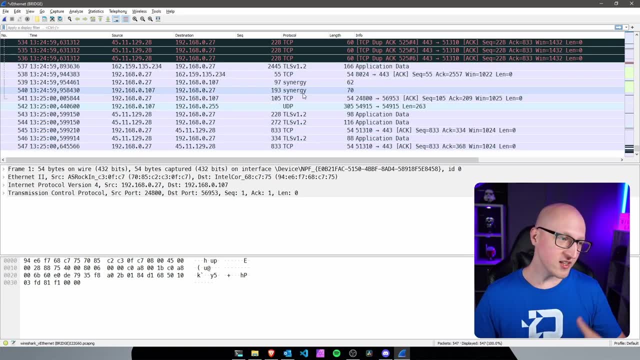 respond with an IPv6 and an IPv4 address. Okay, so let's go back here to Wireshark and let's stop the capture and try to find the DNS request. so you can see, this can be usually hard, right, because there's a lot of stuff going on in the background, but we can also filter here. 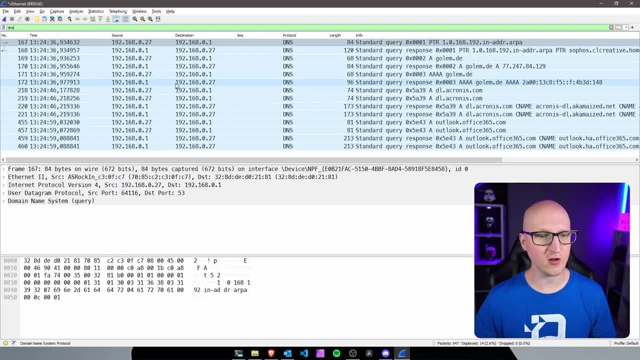 So let's only filter DNS packets, for example, And you can see there are a few DNS requests. my PC has done in that time frame. But if you want to find DNS requests to be more reliable, you can use the DNS server And you can see that the DNS server is also out of the box. This is what my PC has done And 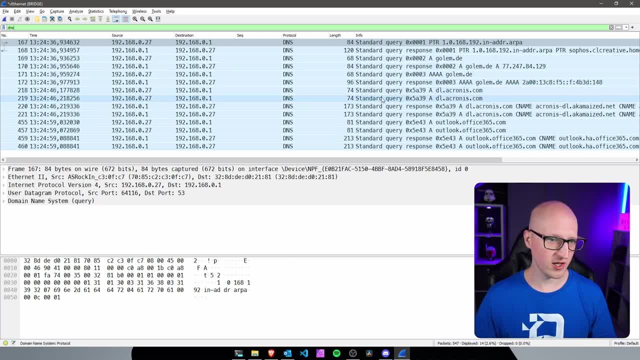 frame when we did the packet capture. so, for example, you can see there is blacroniscom, which may be some telemetry from my Acronis backup software that is running on my pc, or Outlook Office 365 is doing some email stuff or whatever. but we also have our golemde request. 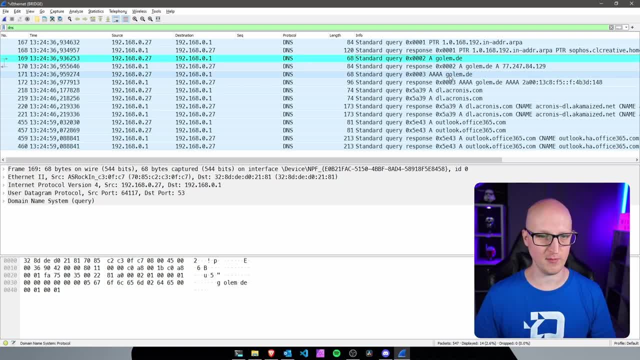 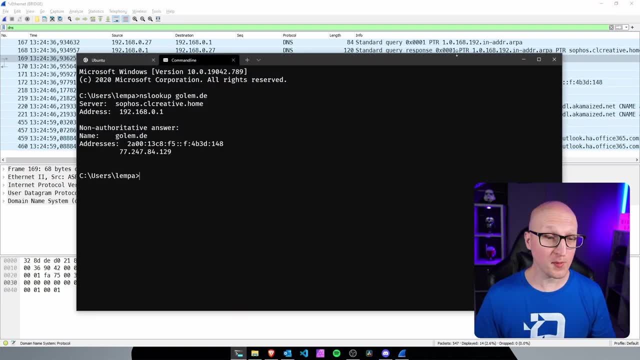 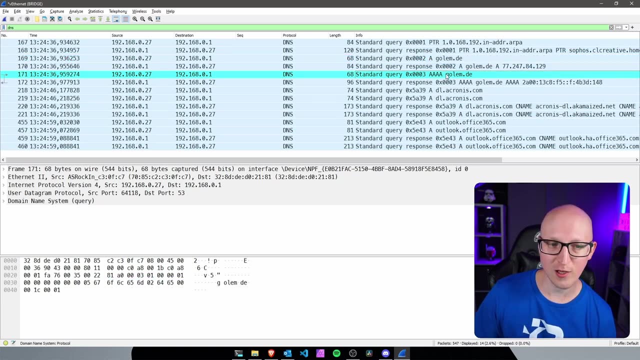 and you can see that we actually have four packets here for golemde. we have two requests and two responses, even though we only did one nslookup, and this is because nslookup will always try to resolve an ipv4 and an ipv6 address, so we have two requests here and two answers. 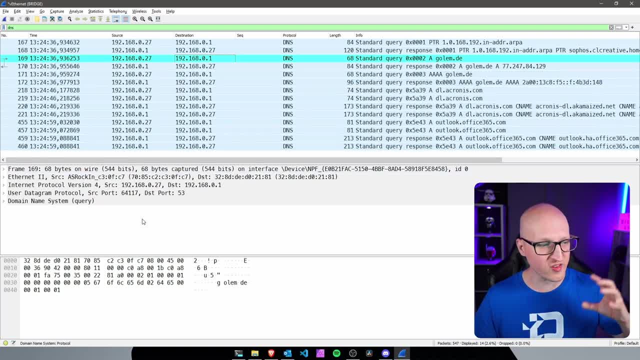 and if we select a specific packet, we can now inspect the raw bytes. but also Wireshark helps us to translate this in a human readable way and when you try to analyze network packets you should always follow the general pattern because they are encapsulated individually: different protocols. these work on different network layers. if you are familiar with the 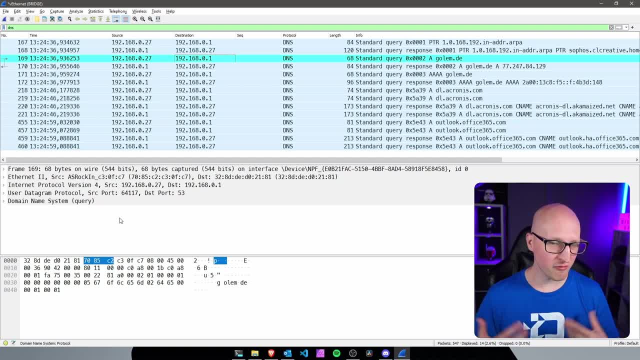 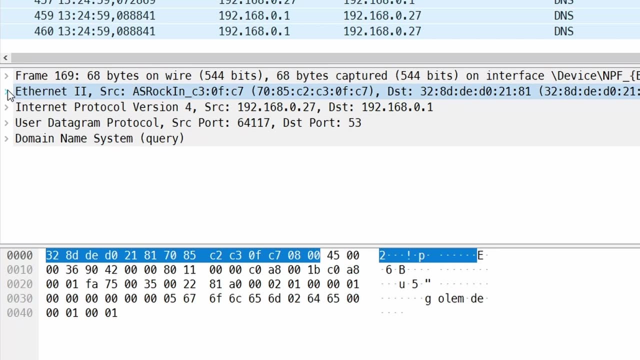 osi model layer 1, 2, 3, 4, 5, 6 and 7. you are very familiar with that. so we always start with the ethernet frame. the physical layer, the preamble stuff and so on, is usually hidden by wireshark. but you always start with the ethernet frame and analyzing this, and here we have the ethernet. 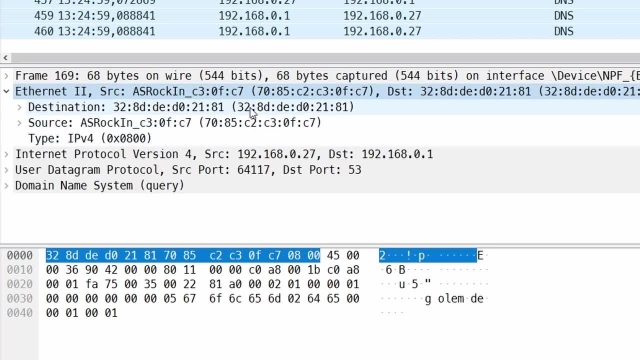 true protocol. so now we are at layer 2. we are talking about MAC addresses. so here is the MAC address to the destination. this is a MAC address from Sophos and also the source address. this is my pc and you can also see. wireshark is smart enough to analyze. it has something like a database. 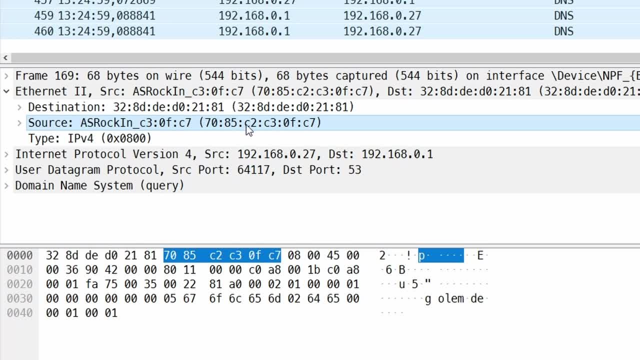 recognizing. okay, this, the first part of the MAC address belongs to the s-rock vendor, so this is my mainboard that i'm using, so it can actually tell. so which kind of network vendor is using these MAC address ranges and wiresharks? help us to identify those kind of things it also has. 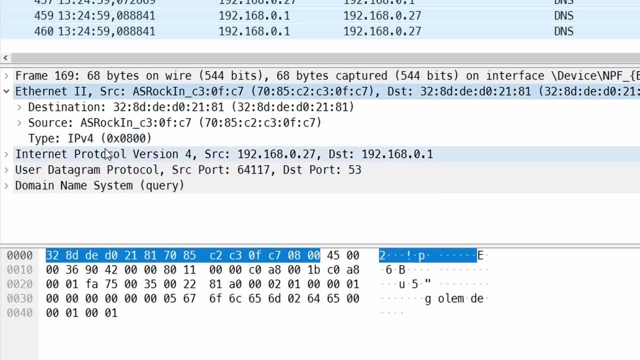 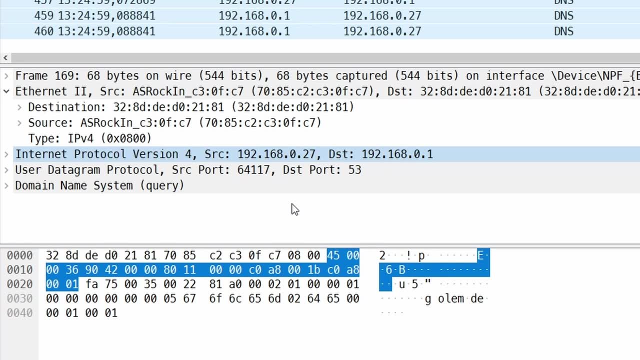 a network address to the destination. this is a MAC address from Sophos and also the source address. so here we have the IPv4 protocol. so that means that everything is in the IPv4 protocol. so when we click on that, wireshark will automatically select those raw bytes where this information is coming. 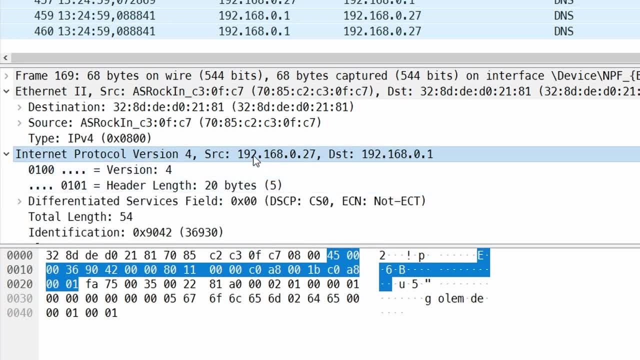 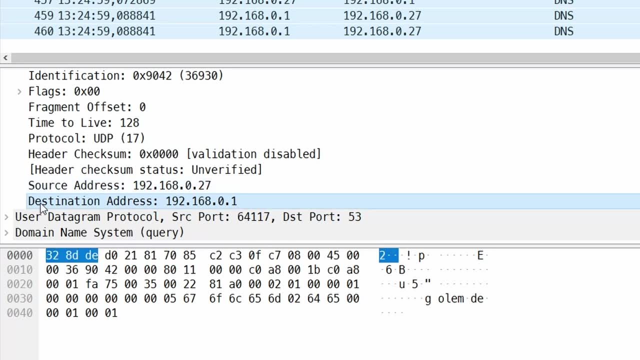 from right and in the IPv4 protocol. we are now talking about layer 3 IP addresses here. so here's the source address and the destination address of my pc and the gateway, and when we go one step further we are taking a look at the UDP protocol. so now we are at layer 4. we are talking about 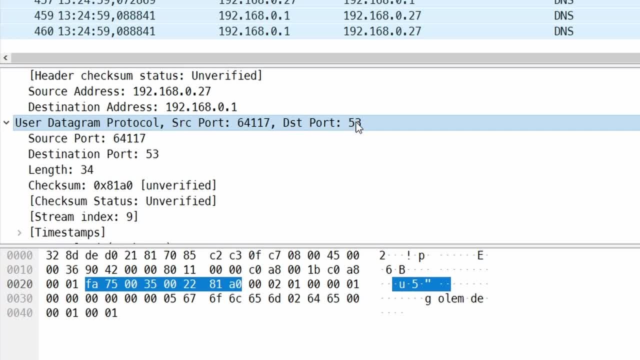 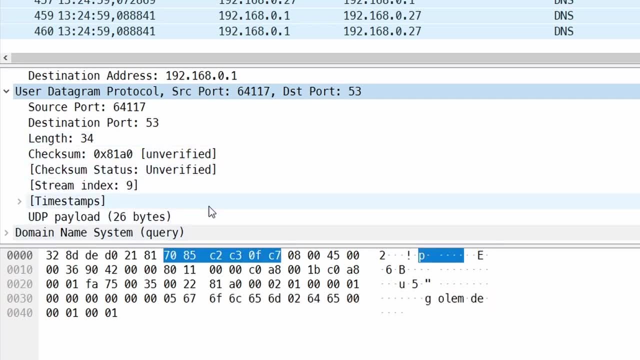 protocols and ports. so the UDP protocol is basically a protocol that allows you to type IPv4 into the MAC address of your MAC address, and the UDP port 53 is reserved for DNS and therefore wireshark knows: okay, this is a DNS request and i need to interpret all this data that is included. 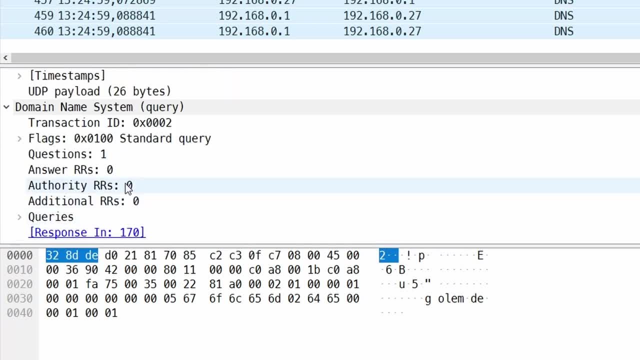 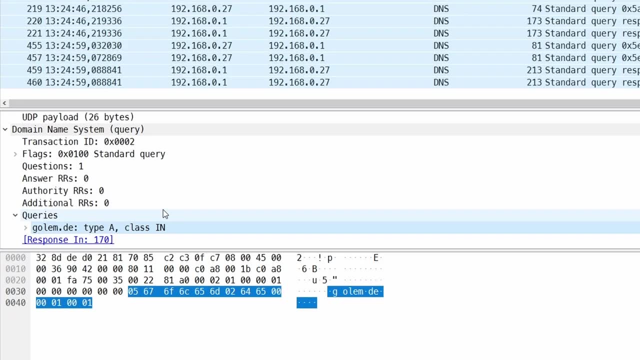 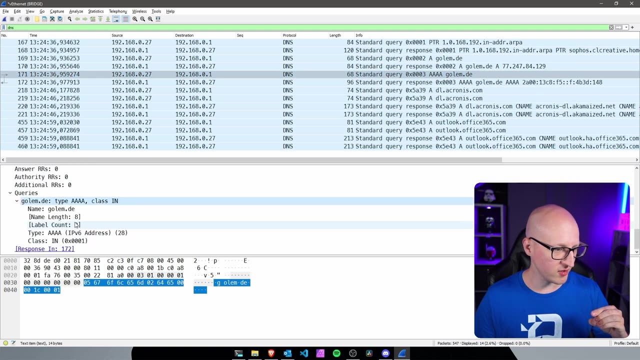 in the packet as a DNS package and when you click on that you can also see there's a query here. our query is to golemde. it is a type a query, which means IPv4. we can also select the corresponding IPv6 request. there's the type a, a, a a, which means IPv6. all right, you can see it here and we also have a. 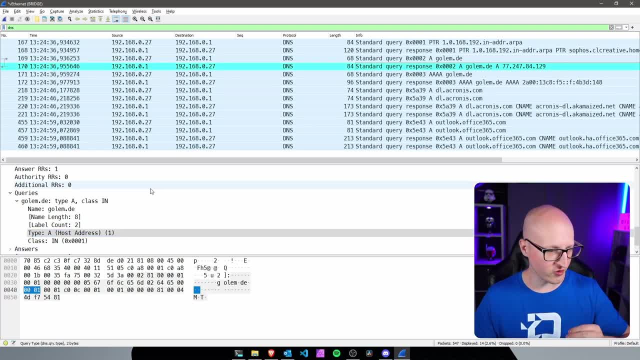 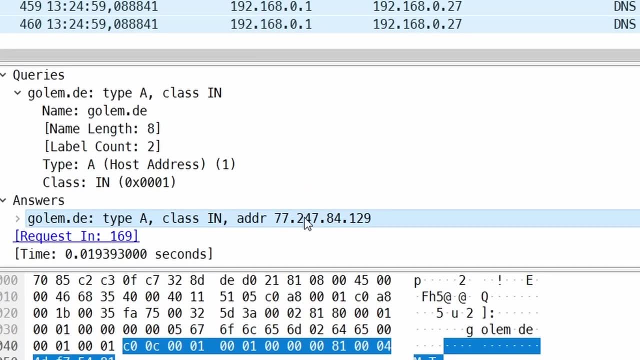 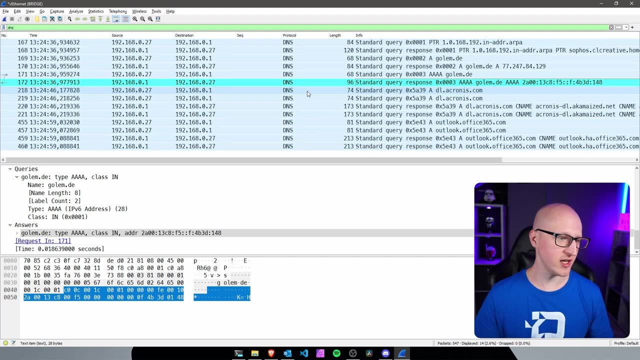 corresponding response from our gateway. this is the first one. this is the IPv4 address. when we scroll down, you can also see the answer here. so that means golemde is at this public IP address and there is the IPv6 address. so this is how you can analyze network packets and you can also 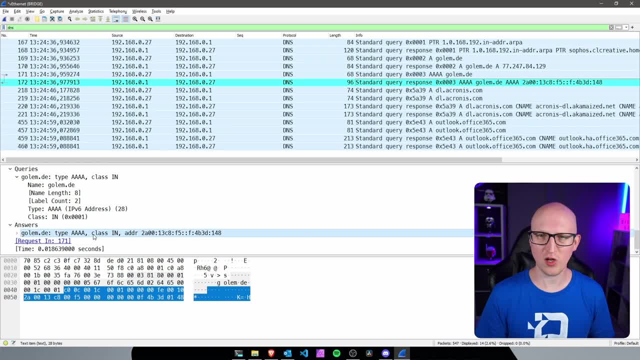 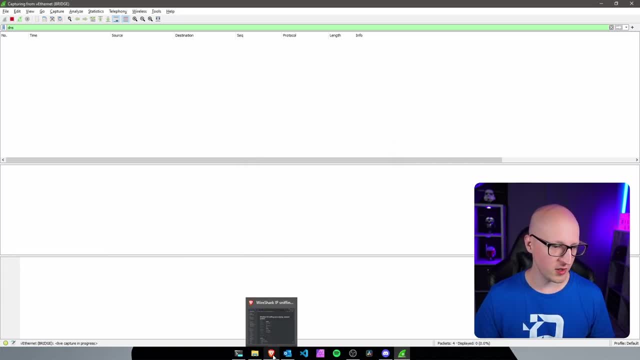 inspect all the data. what is included in the packet? okay, but what about web traffic? let's, for example, try to capture web traffic. so let's do another capture and i will try to open a website. let's open the website, thedigitalivecom, which is a really great blog if you want to become an 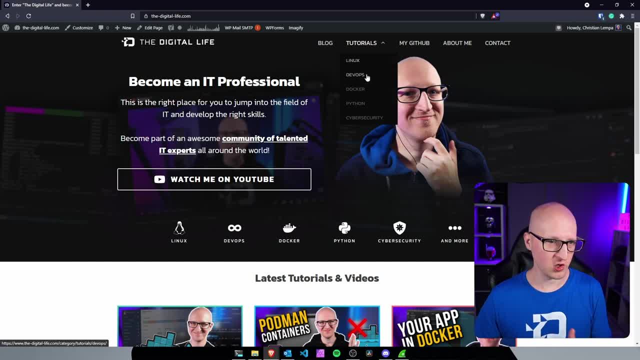 IT professional and you want to learn more about tutorials about linux, devops, docker, python, cybersecurity. read other stuff about me and about my resource and github pages. yeah, there's a lot of great stuff on that home page and because i just did this request, let's go back in wireshark stop. 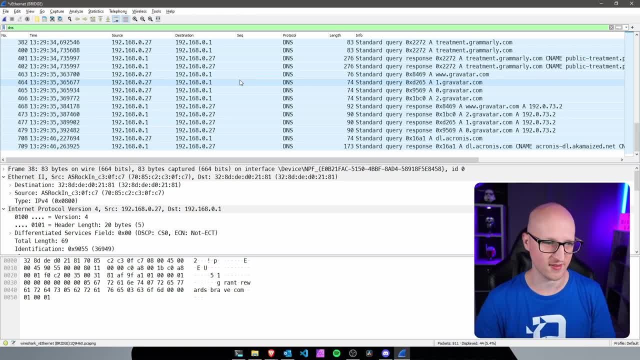 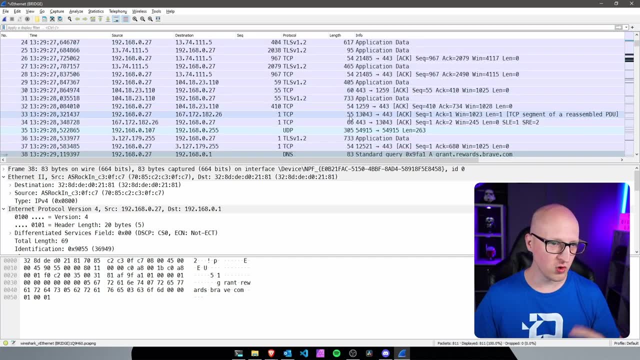 the packet capture and let's try to find the https packets. now we can still only see the DNS packets. this is because the DNS filter is still active. so click on that x to move that filter and now we see all the packets that have been captured. you can see there's a. 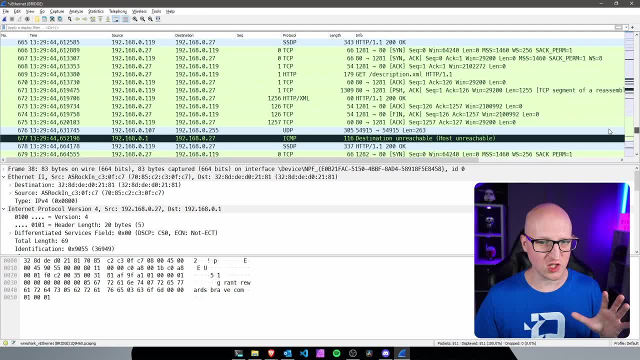 lot of stuff going on there and it can be quite hard to find the https packets. you can also see there is something like an http. this is unencrypted traffic, so this is a great example. let's first of all take a look at this here. i don't know what that is, but http traffic is unencrypted, so we 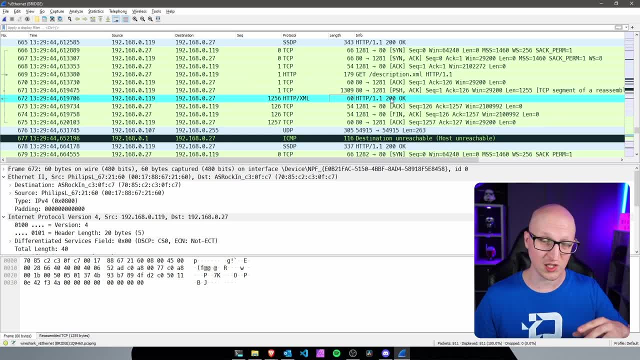 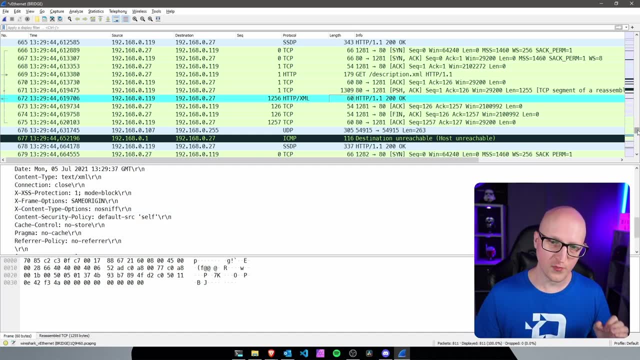 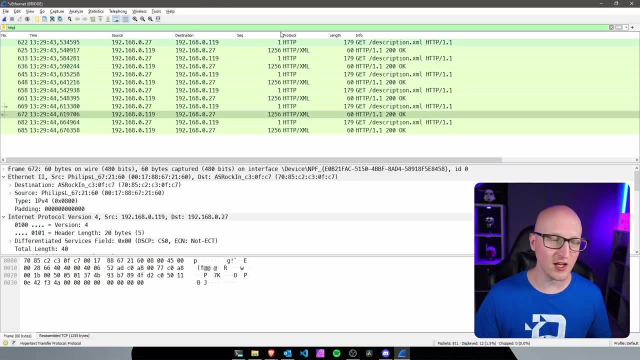 are able to see all the data. we are seeing the http request and the response with the 200. okay, and we can actually see the data. but anyway, let's search for our https request. so now we can filter based on http, but then we only see the http and not the https. 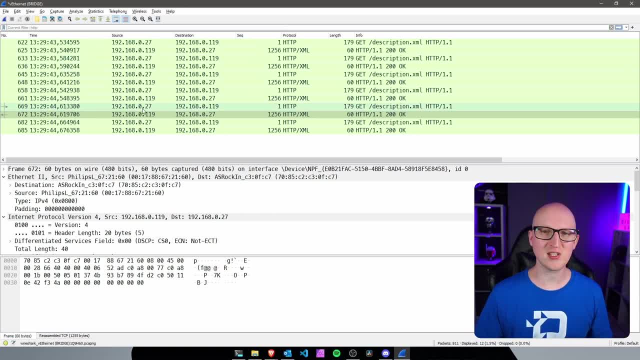 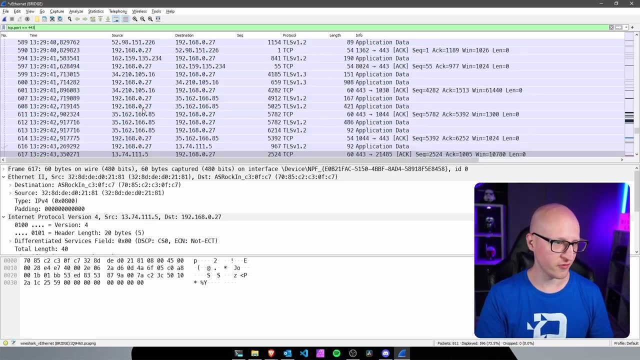 request. so how can we filter on that? we could basically filter by port, because you probably should know that https operates on the tcp protocol on port 443, so mainly search for the protocol, tcp and search for port is equal, equal, 443. so now we only see https connections that are operating on 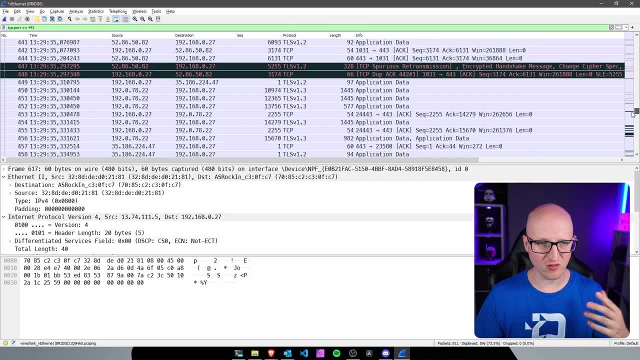 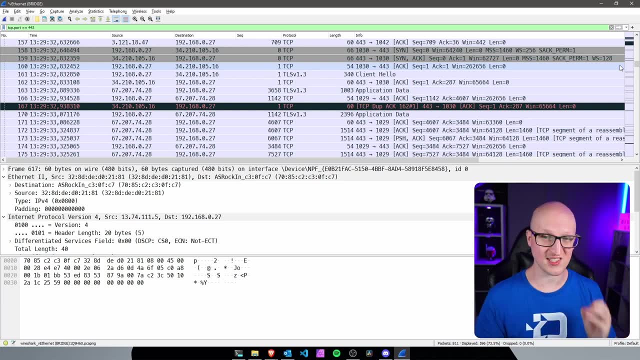 port regularly and we can all scroll up and try to find our specific requests. you can search for different things here and i will show you how to identify the specific requests, even though the data is encrypted and we don't see the html code inside these packets, but an https request always. 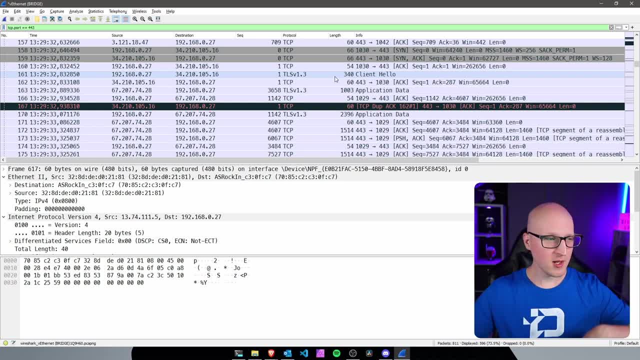 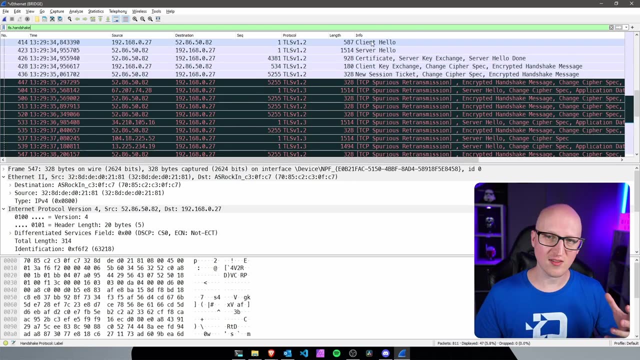 starts with a client hello and the client hello is part of the handshake that the client does with the server, so they do something like an ssl key exchange and all this stuff, right, so we can always see what the client is doing and we can also see what the client is doing inside the client hello. 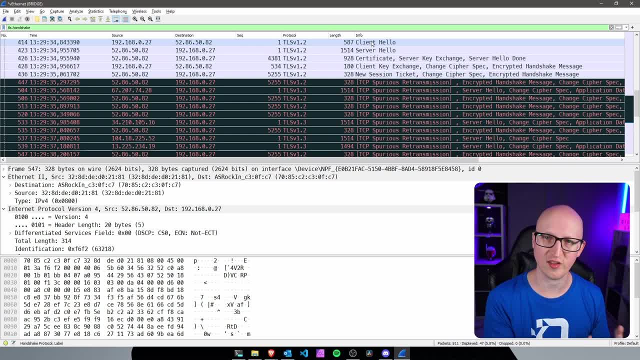 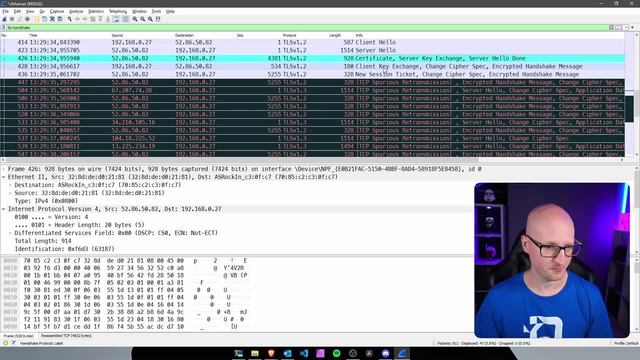 and this is the tls handshake, for example. so let's apply this filter and then we only see packets that are part of handshake processes from the tls protocol. for example, a client in a server, hello, the certificate and the key exchange. that's happening here. although all this traffic here. 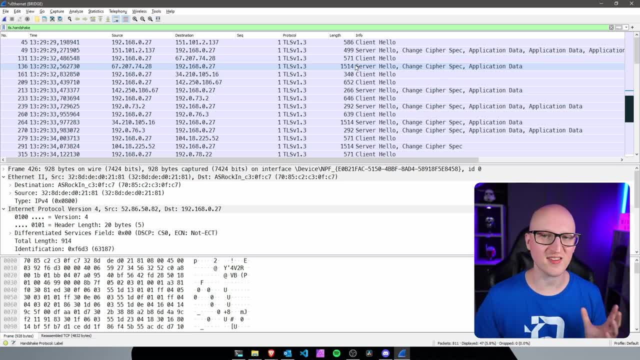 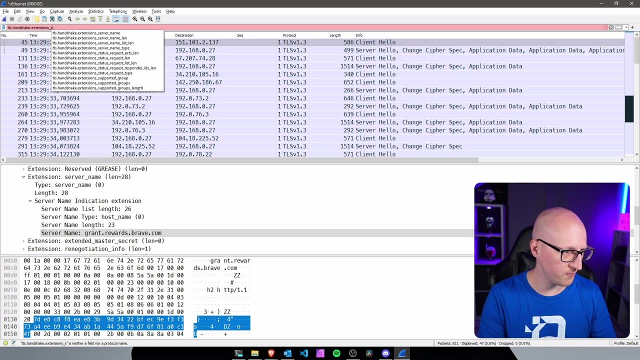 is encrypted. there's one particular part that is still unencrypted inside the client hello and this is the sni, the server name identifier, and we can also filter by that. so let's try to search for tls handshake, because included in the handshake, and then extensions underscore server name, so the server name and then we can search for. 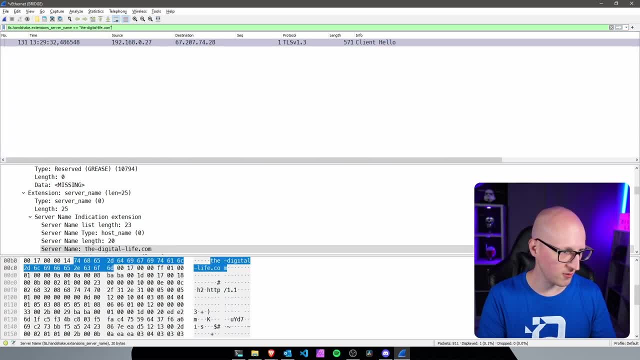 a text that digital livecom. and now we get our specific client. hello, the request that our client does to the digital live web page and you can see the information is unencrypted in here. so anyone sitting between your pc and the network traffic, maybe at a gateway or anywhere in the network in. 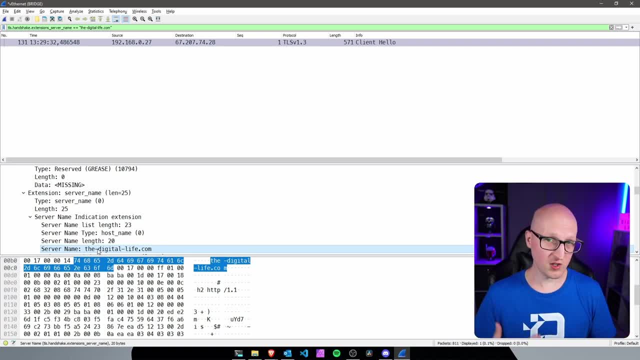 between can actually see which websites you're browsing. maybe some of you didn't know that. okay, so let's take a look how we can actually see all the traffics that are corresponding to that particular connection, because all the requests are separate connections. so now in Wireshark we 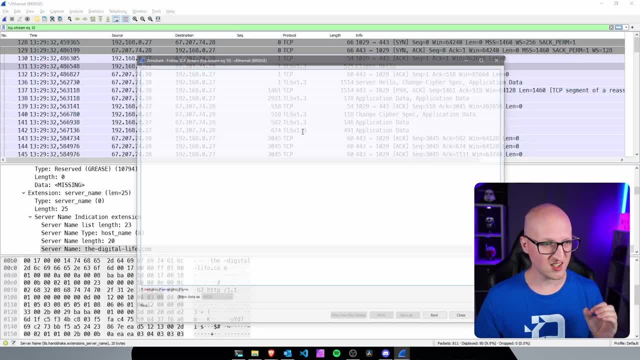 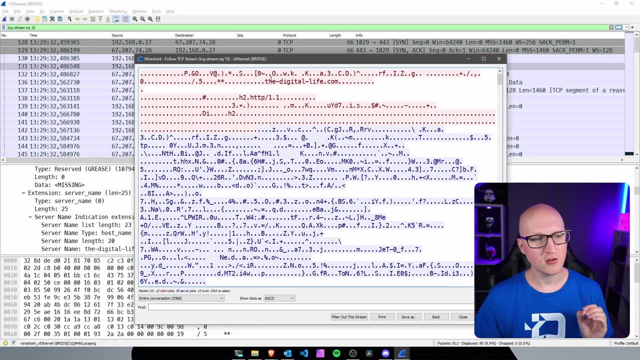 can use something like this here: we do a right click and select follow tcp stream. so now we get all the information, the whole TCP stream requests that my PC was doing. you can see it is going to the digitalifecom and it is an HTTP 1.1 protocol request. but then all this information that comes. 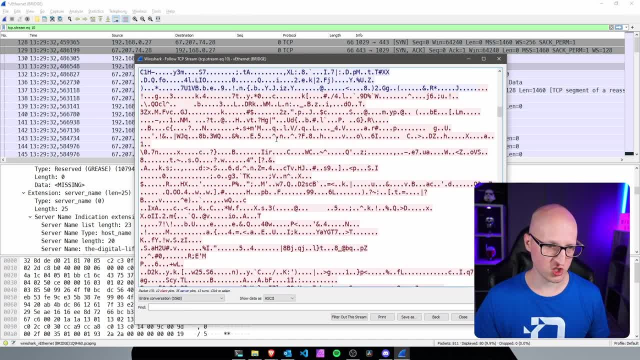 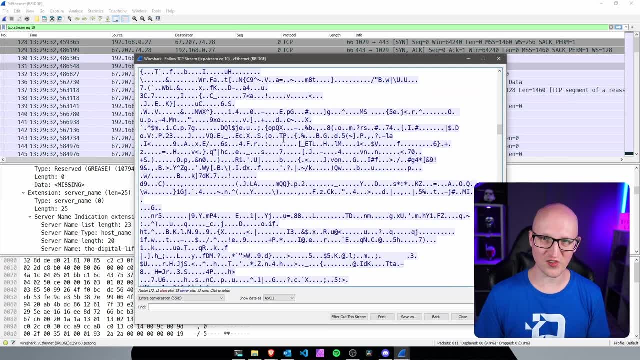 here- that is, usually the data- is encrypted information so we can see inside the HTML code or can inspect any passwords or anything like this. so that is a good news, right, even though you can always read the URL, because you can inspect the SNI and encrypted web traffic. you. 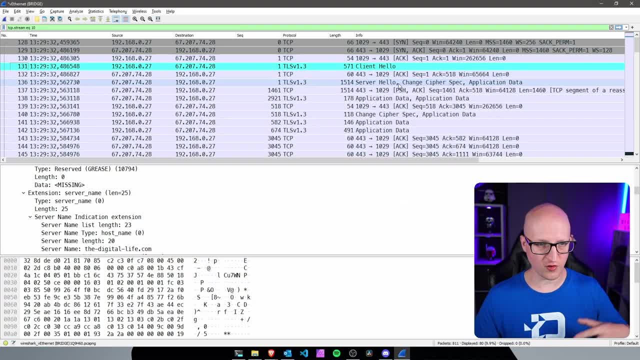 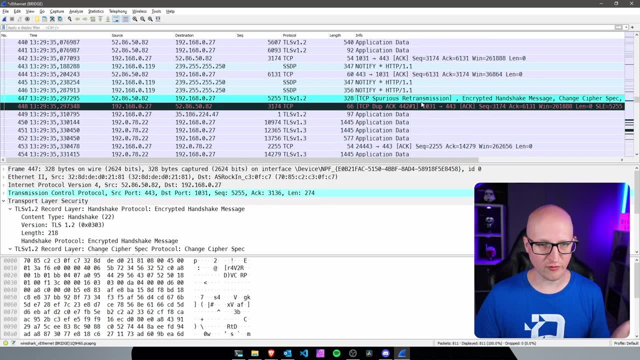 can't see the data okay. so I hope this was quite interesting and you can also analyze what is going on. I will also show you something else. so, for example, if we scroll down here, you may see some retransmission here, for example, this year, the encrypted handshake messages. we also see duplicate 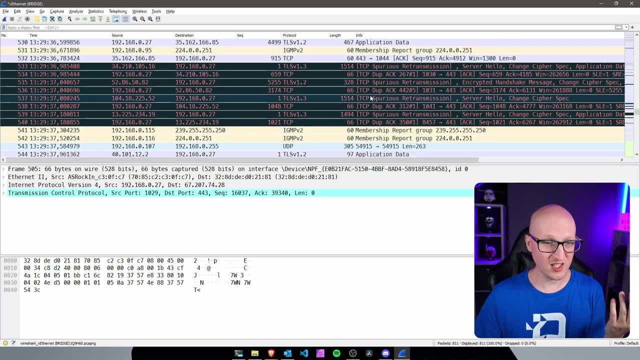 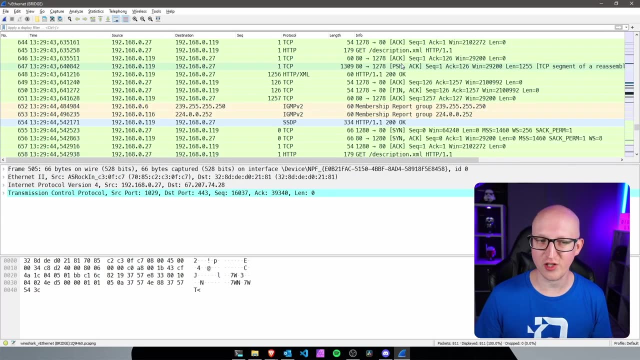 acknowledges here spurious retransmissions and there's even more stuff going wrong. so this is something you usually see in network traffic. so there are always things going wrong, there are always packets that are missing, and this is because the network protocols always have issues. right, especially in wireless networks are much more. 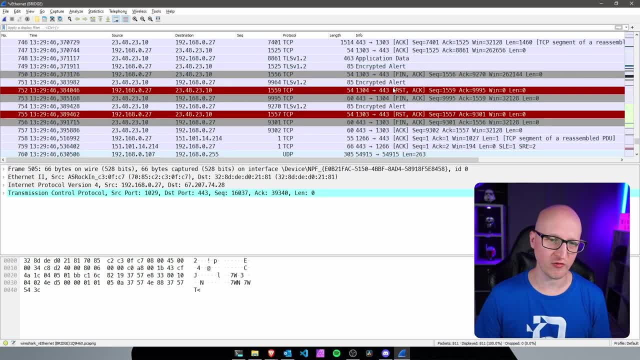 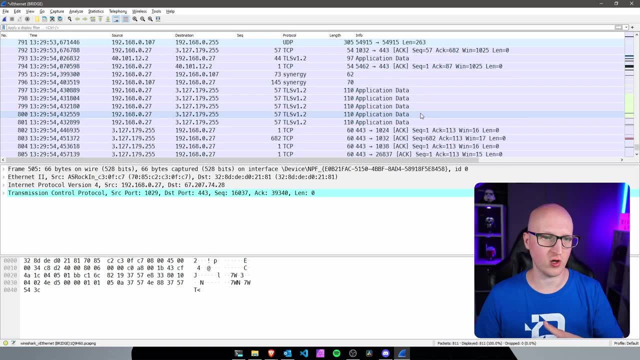 errors happening and this is kind of normal. this is nothing you should be worried about. but if you're really trying to find out what's going wrong and you're seeing a lot of retransmissions or maybe some other issues happening inside the network, packet something like this here and you always 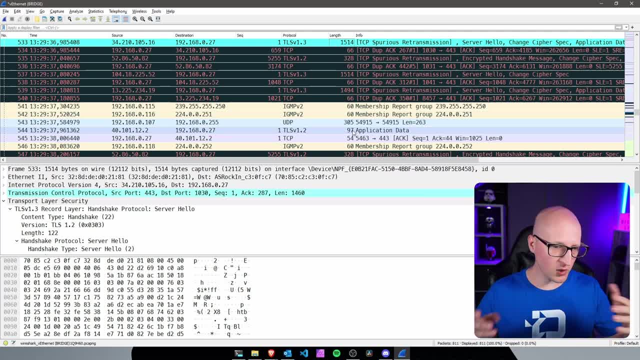 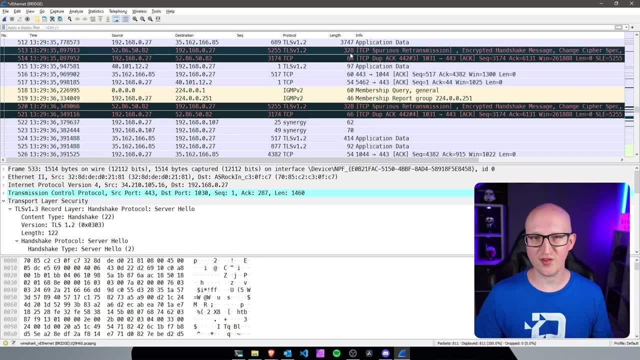 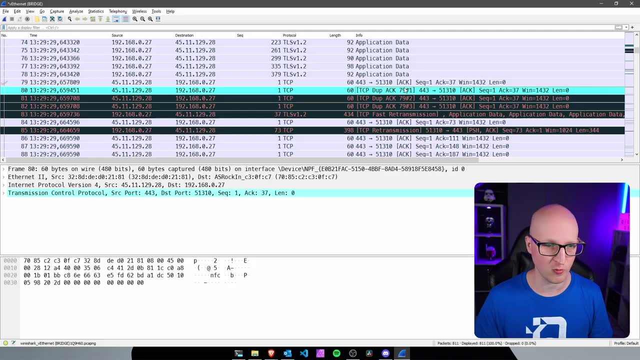 see black and red colors, then something is going wrong and you probably want to take a closer look into that and try to find out what's going wrong. so in the TCP protocol you will always see messages like this here, where the client or the server has requested to retransmit specific network packets that have been lost on the wire. so 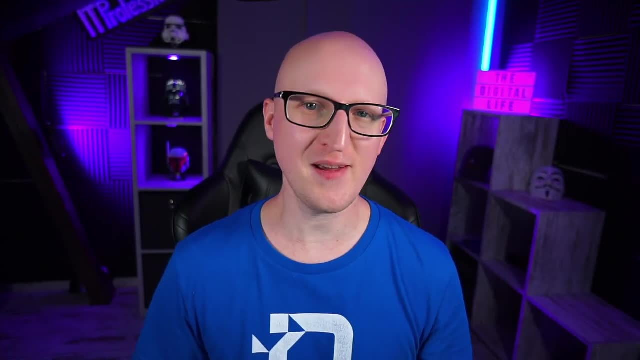 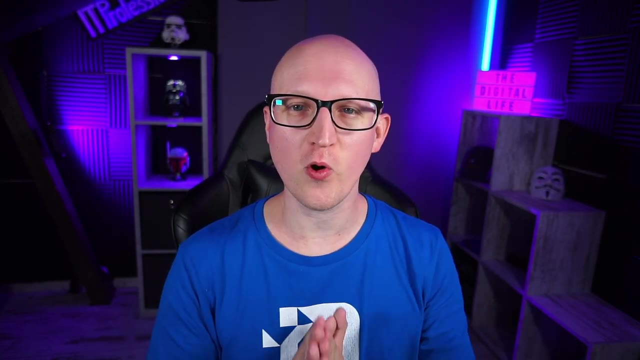 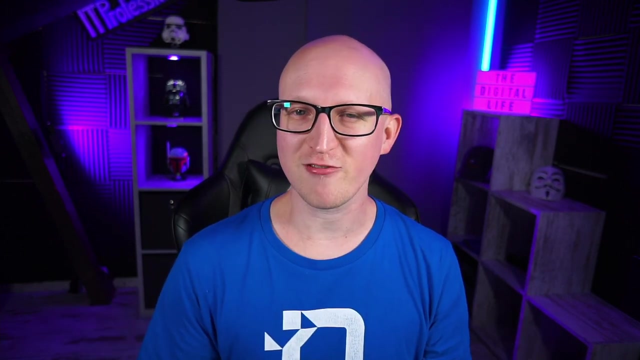 you can see, Wireshark is an extremely powerful network tool. I mainly use it for studying IT certifications, do researching or just troubleshoot issues and, as I initially said, if you're working in a computer network where you have many devices like servers, Gateway switches or whatever, you may want to capture network traffic, not just on your local. 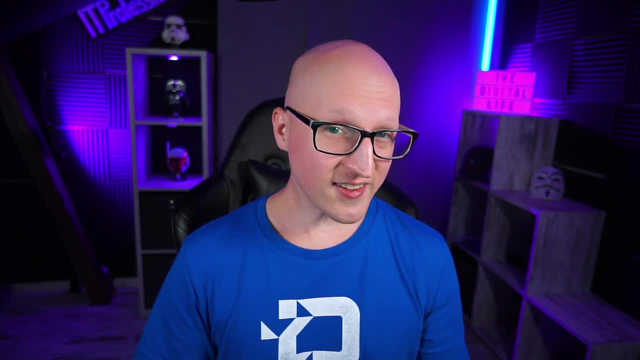 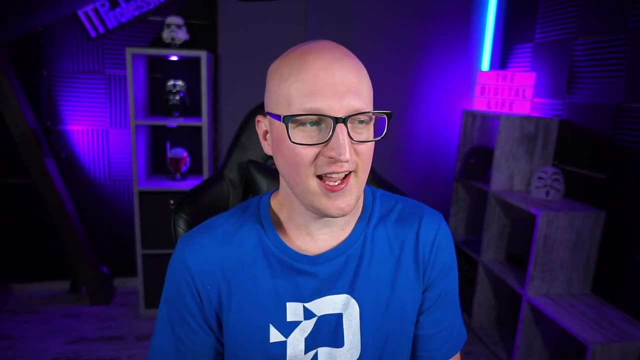 PC, but also on a remote server as well. so in this case you can't use Wireshark for capturing the traffic, because it is just running on your local PC. on Windows servers you probably can install Wireshark, of course, but on Linux servers, where you don't have a graphical user interface, but you still. 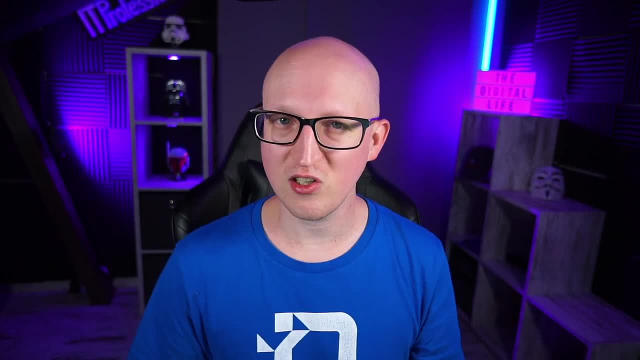 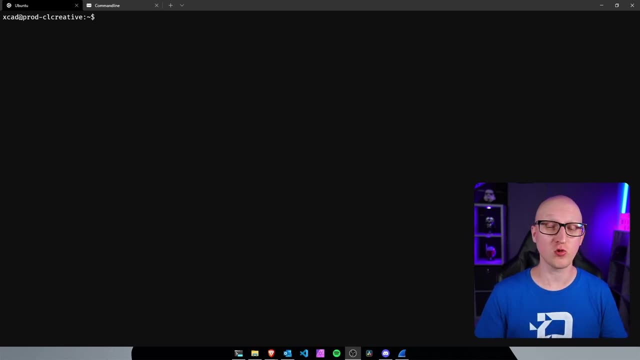 want to be able to capture those traffics. there is another possibility to do that, and I will show you a scenario. for example, I'm now connected to one of my cloud instances and my cloud instance is connected through a VPN with my local PC. I'm using tailscale for doing this, because tailscale is a 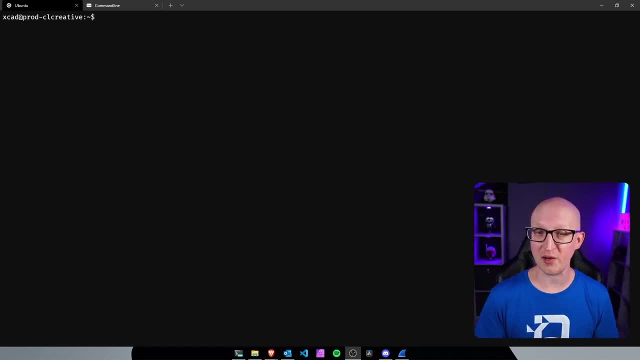 very great and easy way to use something like a managed VPN provider that is powered by WireGuard. so I've made a tutorial about tailscale, and if you want to learn more about this, just check out the link in the description down below. it's really an awesome tool. so tailscale is now connected to my 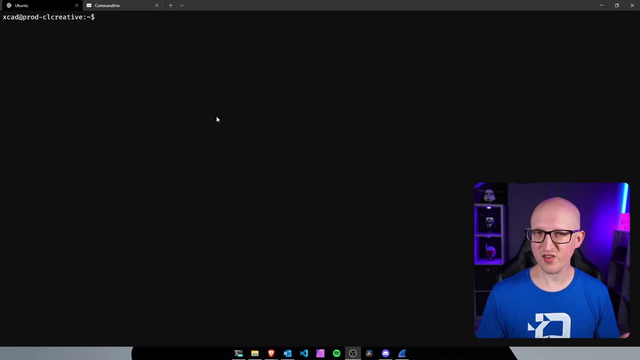 cloud instance and my local PC and I just want to show you how to do that. so I'm going to show you how to run a simple web server here to just capture a request and, for example, I want to run a simple Docker container that is running an unencrypted web server here, but only in the range of my local. 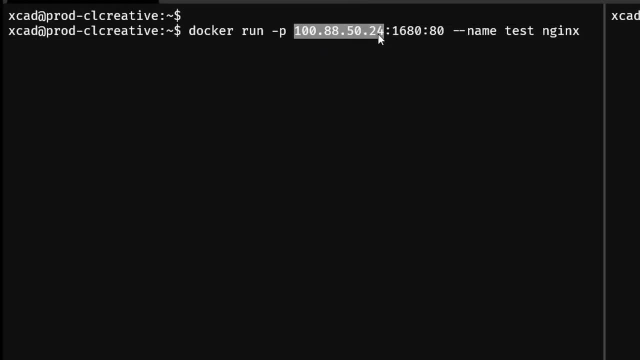 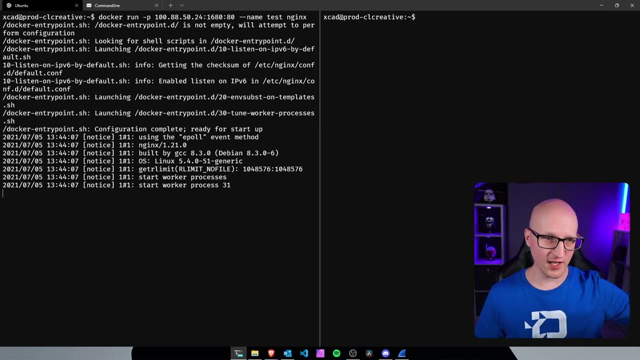 network. so I'm just limiting the access to this particular private IP address and I want to be able to capture the packets that are coming from my local PC to my cloud instance on that particular IP address here and I want to capture the packets on the cloud server itself because I 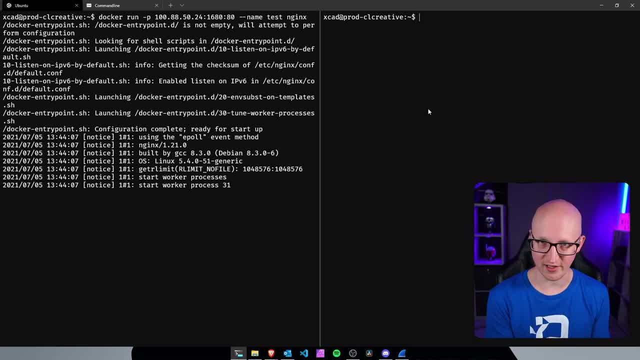 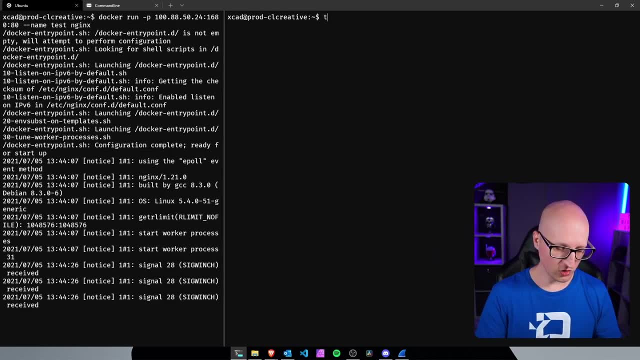 know if the web request is hitting that server. So to capture the network packets on a cloud server, I want to use a tool that is called TCP dump. So TCP dump is a tool that is very similar to Wireshark, but it doesn't have a graphical user interface. It simply just does a packet capture. 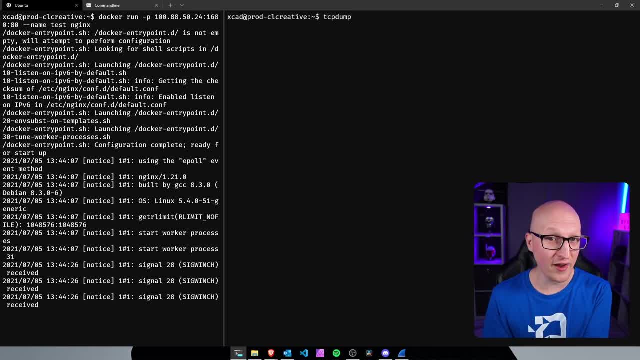 but it is able to save that packet capture to a text-based file And you can later download this file and analyze in Wireshark. So let's do a TCP dump And I first of all want to specify a specific interface, just like in Wireshark, So with the dash I parameter I want to select an. 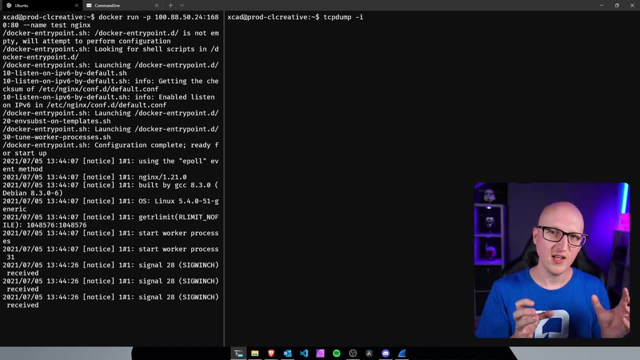 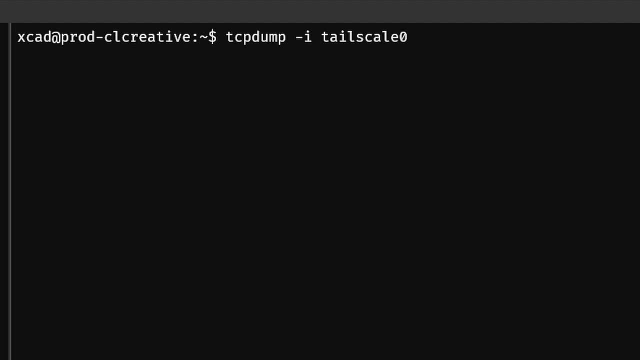 interface And in my case I want to capture the packets that are not hitting my public interface but my internal VPN interface, because I want to see the packets that are unencrypted there. So detail scale zero is the internal VPN interface. I want to do the packet capture on. 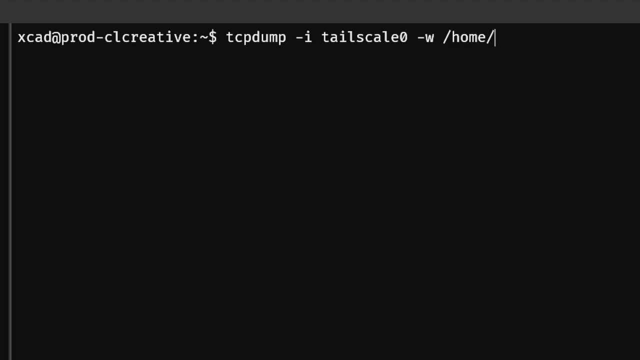 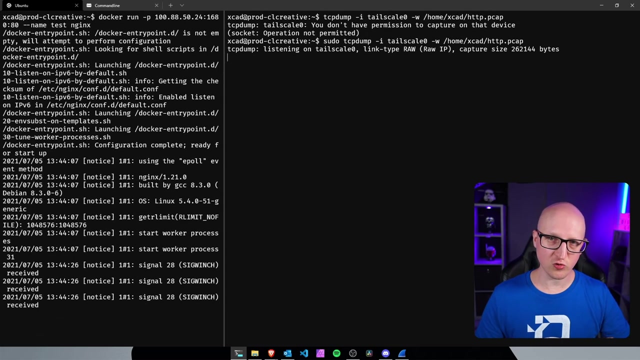 And I want to write this to a file that is located in my home folder and just call it httppcap, and pcap stands for the packet capture file format. so let's do this, and i need azure permissions, of course. and now i want to try to initialize an http connection from my local pc. 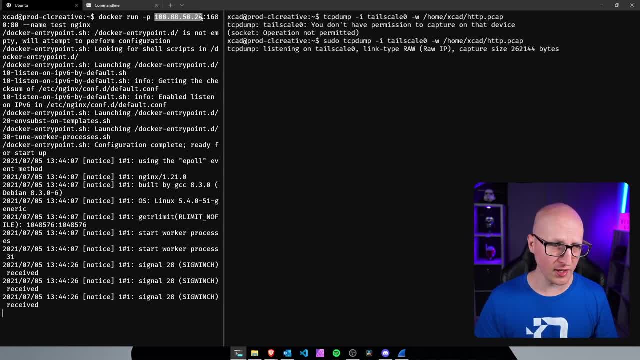 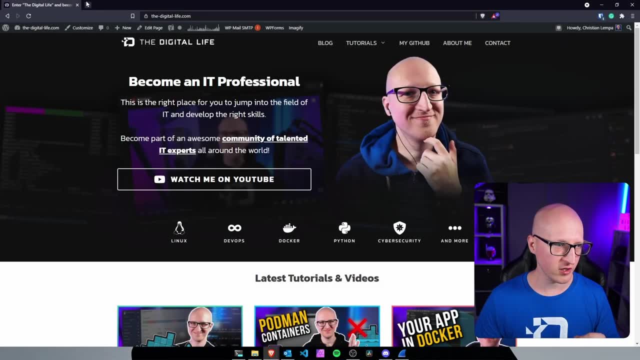 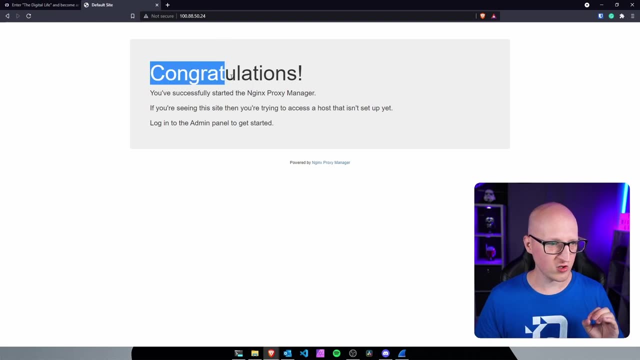 to that cloud server. so because i'm connected to my vpn, i simply can just execute this web request on that private ip address. so let's open another browser tab and do http on this ip address and if i hit enter, congratulations. you are now running the nginx proxy manager. so you can see, that is something different. let me just go back. 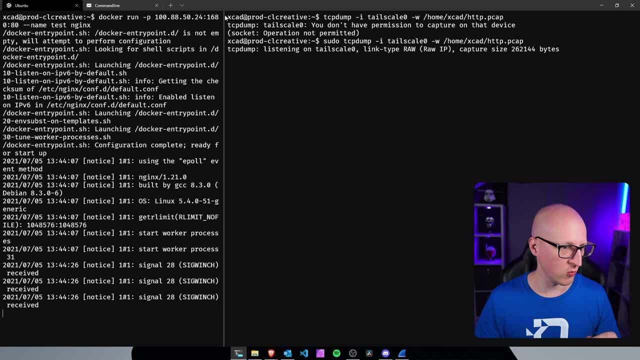 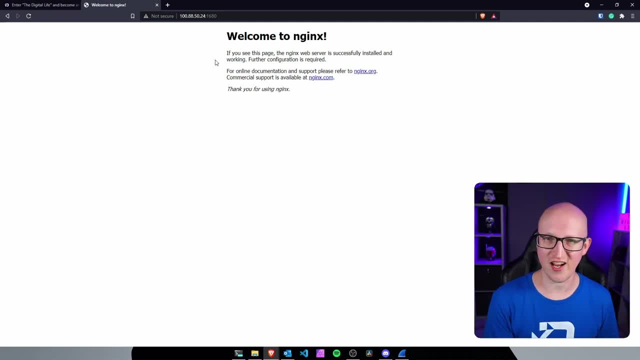 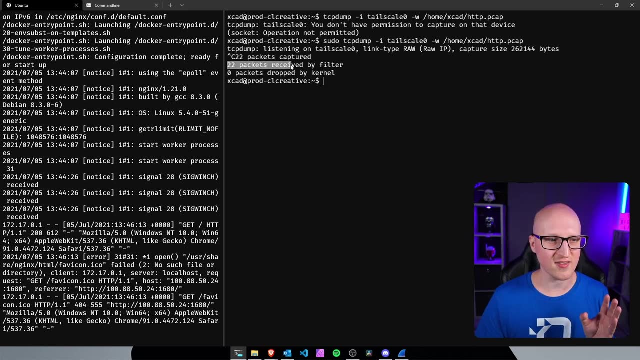 ah, yeah, so i have used another port, that is uh 1680, so let's do another request here to this particular port, and this is a web request to our nginx web server. when we go back here and we stop their packet capture on our remote server, we can see that 22 packets have been received by the filter. 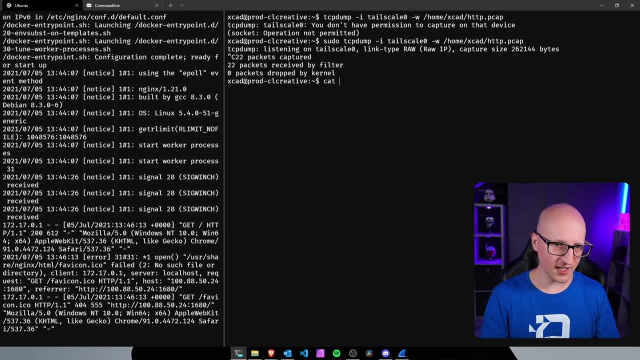 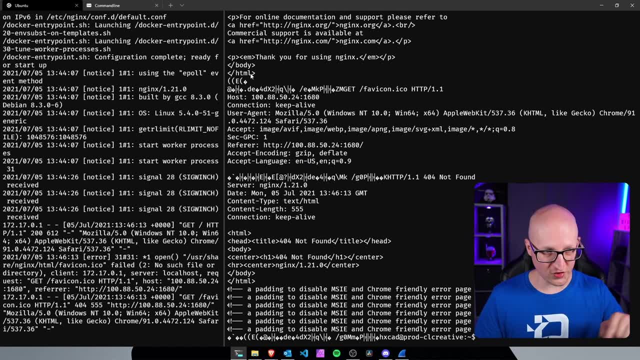 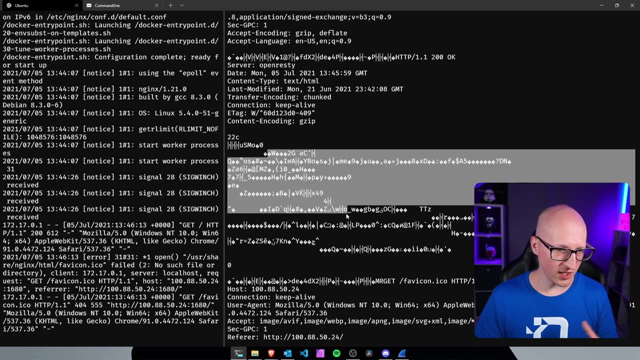 and they are now stored in that file. so when we cut that file, you can see that everything is in a text-based format. it is the rare packets, but you can also see some html code inside here, because everything is captured right, but there's still some stuff that you're not able to see correctly. 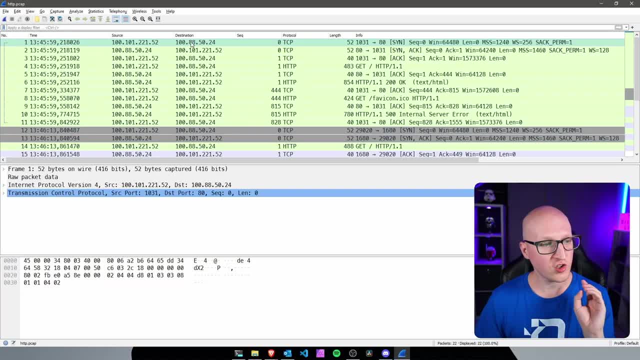 so let's download this file and open it in wireshark so we can see the destination, the private ip address. and here's a private ip address of my windows pc that is connected via the tailscale vpn and because we are capturing on that vpn interface and not on the external interface, we're able to see all the. 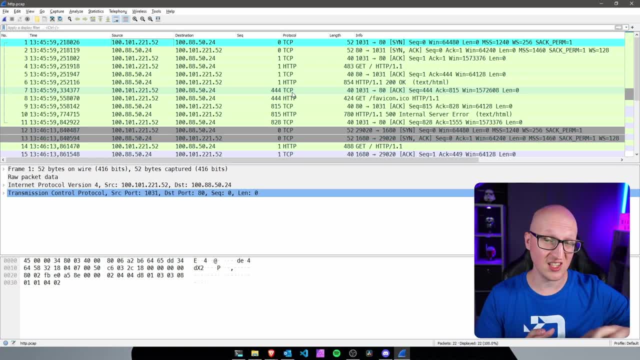 packets that are inside the vpn tunnel and we are seeing them unencrypted right because we have captured this at the internal vpn interface. so this is very important to understand where you're capturing this, what you want to see and when we go here and follow this tcp stream. 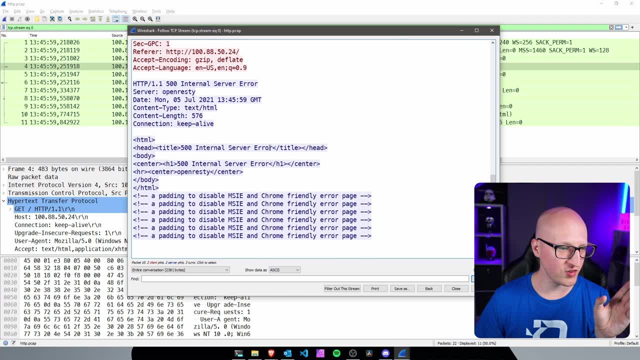 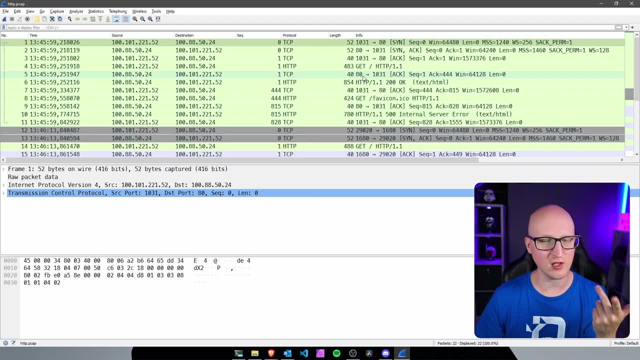 we can see the full rack request that we have done and we also also see our internal server message. so this is probably the nginx proxy manager. remember, i've done the real web request at a different port, so let's scroll down. so this is a real request, not. 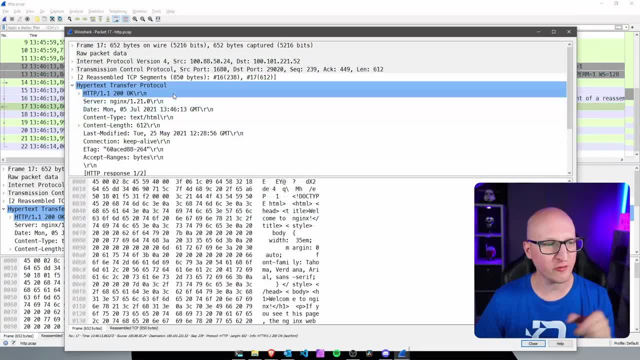 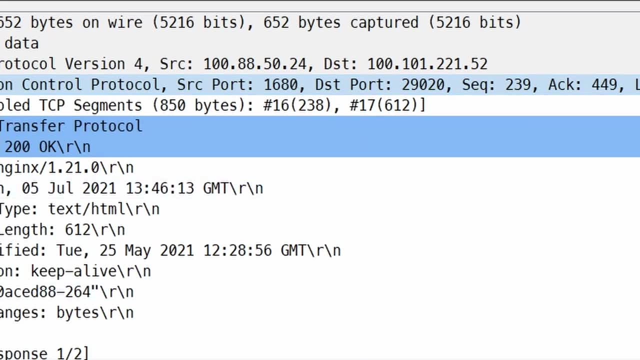 to the nginx proxy manager. this is the second one and we can differentiate that by the source port that remember i've used the port 1680 to make this request and if we now follow this second connection, we can actually see that there is our html code. 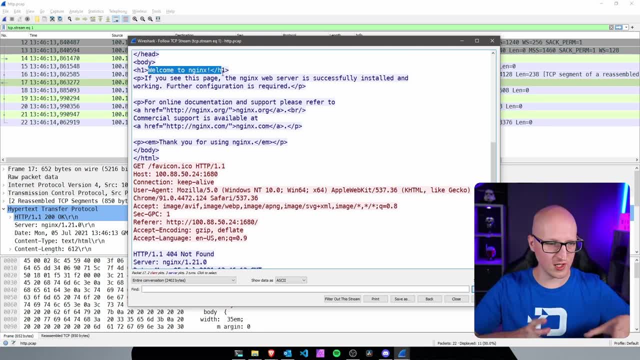 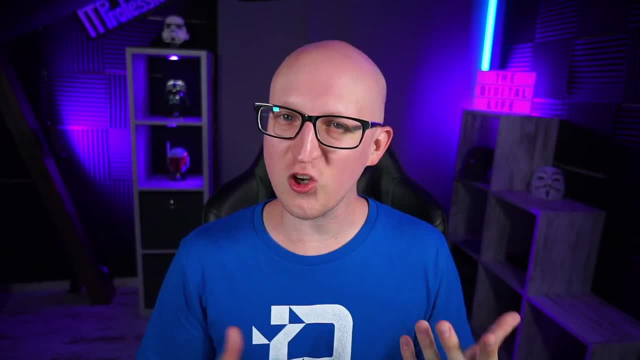 for online documentation. this is welcome to nginx. so this is our real web request and we can now use that to analyze it or do some troubleshooting, whatever is going wrong. okay, so this is really quick what you can do with wireshark. i know you can do so much more with it. 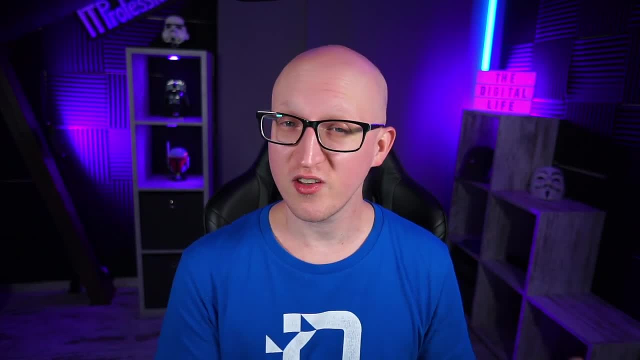 but this was just a short presentation on how i've used this tool to troubleshoot network traffic or to find out whether specific traffic is hitting my servers or going through a vpn or whatever. so please tell me which tools are you using, so what is your experience with it and if you enjoyed. 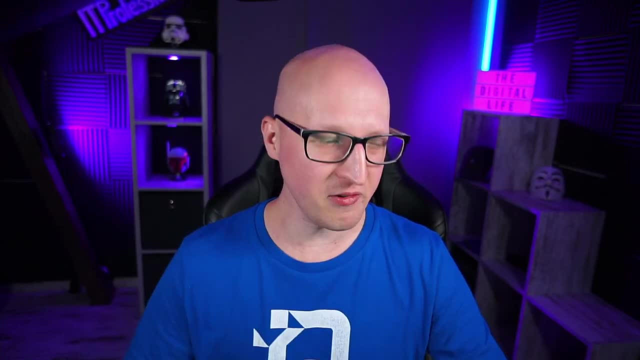 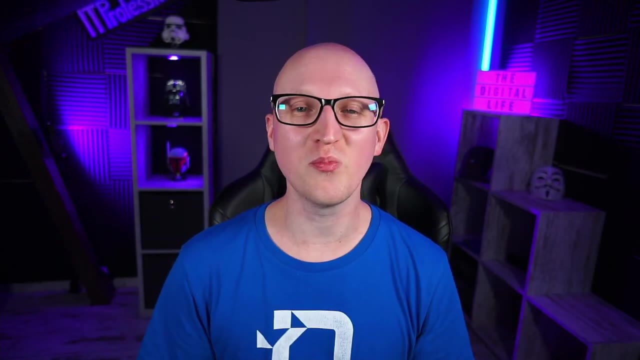 video. please don't forget to hit the like button and, of course, subscribe. if you want to watch more tutorials and content for it professionals, and if you want to support my channel even more, then just sign up to my new youtube membership program. okay, guys. so thanks everybody for watching and as 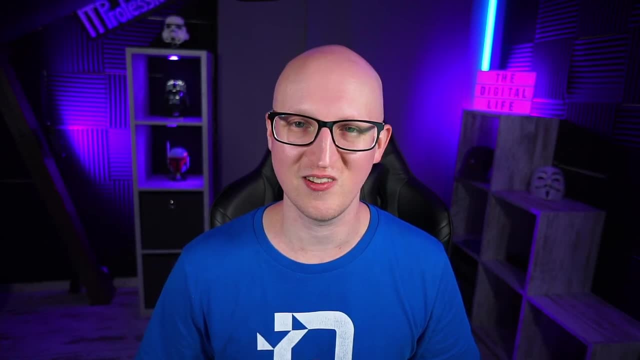 always enjoy the rest of your day, take care of yourself, and i see you in the next video. bye, bye. 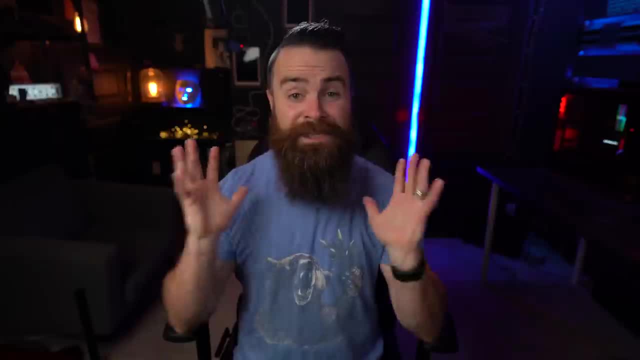 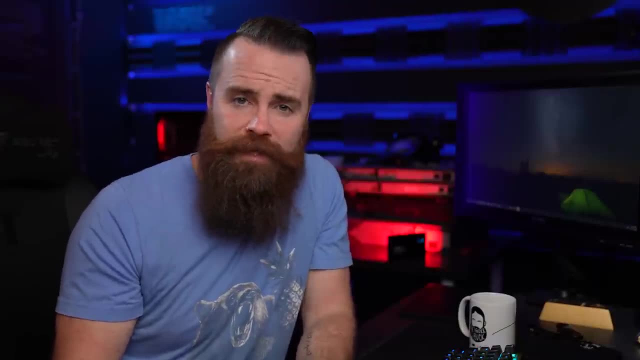 Sequel, It's more than an injection: Get out of here. It's the love language of our databases. You know the massive Excel spreadsheets that run the world. You need to learn sequel, Probably right now, especially if you want this job, or this job, or this job.